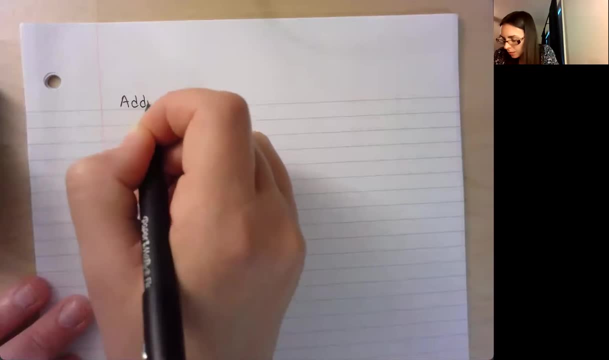 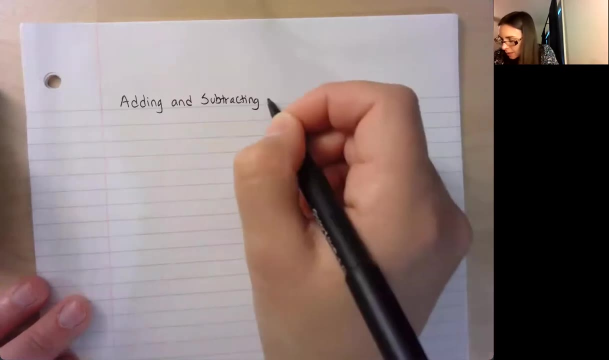 So we're going to be adding and subtracting 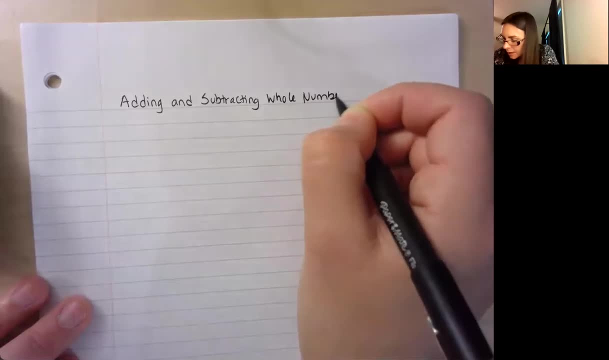 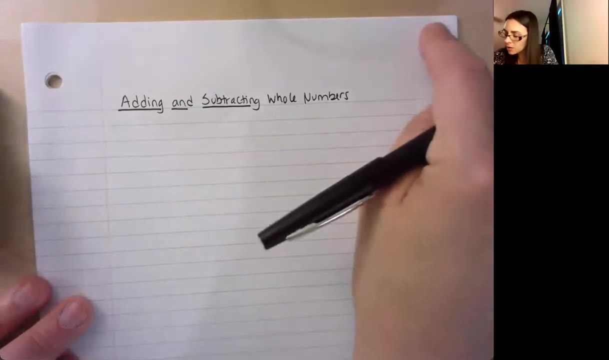 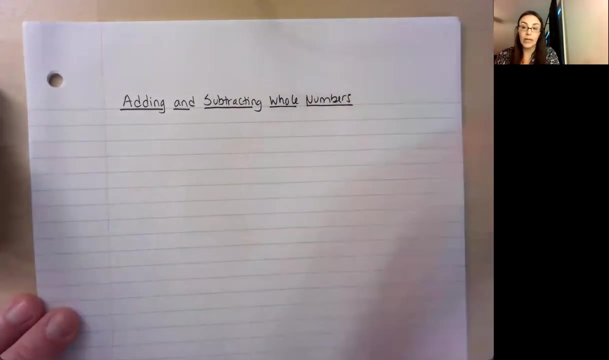 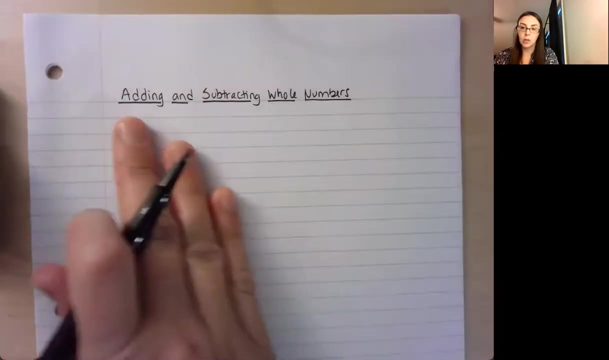 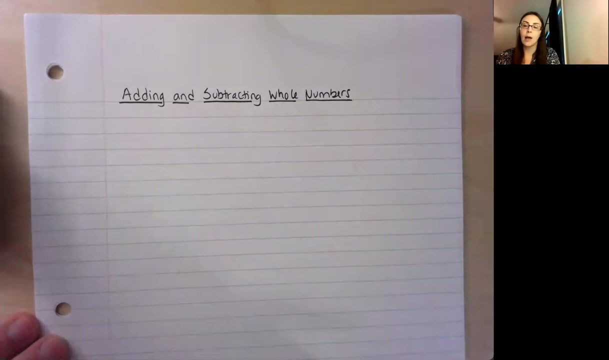 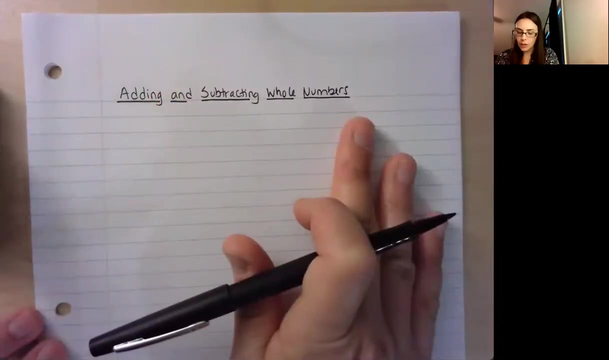 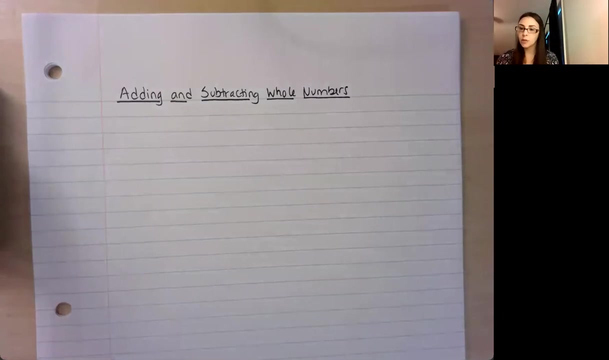 numbers. Now at home, again, I do also recommend you put the date in. So I would maybe write the date right here or at the top, just somewhere, just to help you stay organized so that you remember when you actually watched this or which week the material was from, for instance. So that could be really helpful, too. So you definitely want your title, and you want ideally a date or maybe, you know, what week you're learning this in and so on. I also recommend when you do your notes, starting each subject on a new page. I know some students like to save paper, and I do agree with that. So they'll maybe continue it underneath another topic. But if you find that too confusing, just flip to the next side or the next sheet and start your new topic up top. So today, we're going to be talking about adding and subtracting whole numbers. And again, hopefully, this will be a review for you guys. But if not, that's okay. Take some good notes like we're going to do here. So what I write down, you want to make sure you write down. You can also write down extra, 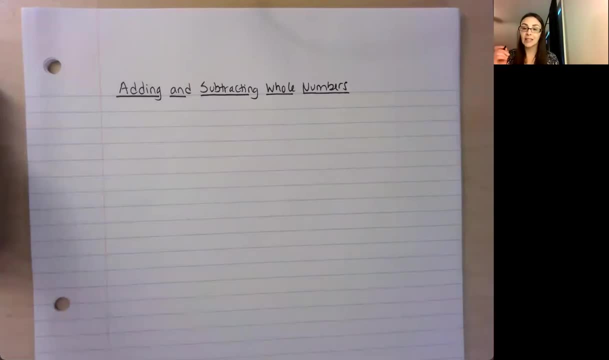 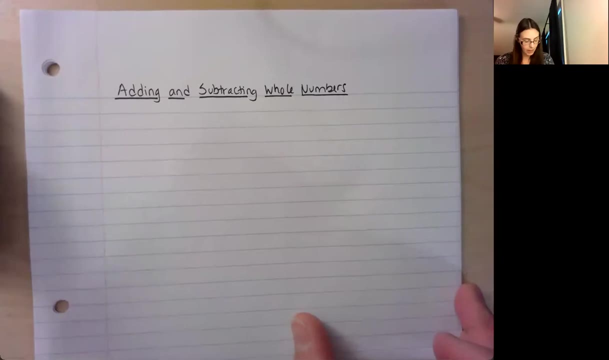 so if you find that you need to fill in some gaps or add some more notes along the way, definitely do that, too. Okay. So just a couple key words here first before we start. 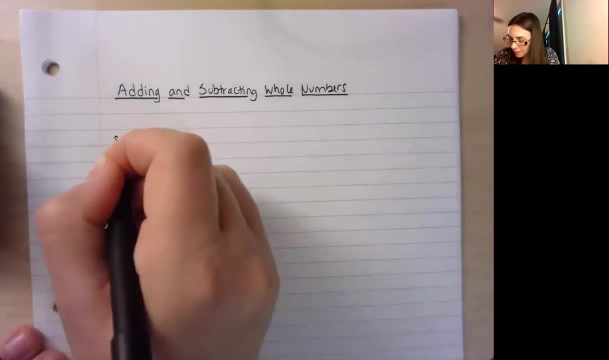 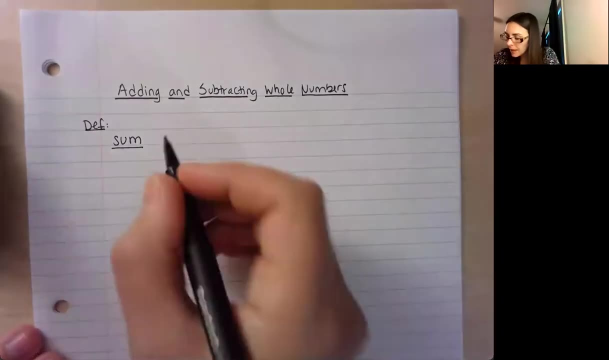 So our first key word is a sum. So maybe we'll just write some definitions here. And the word sum is the answer 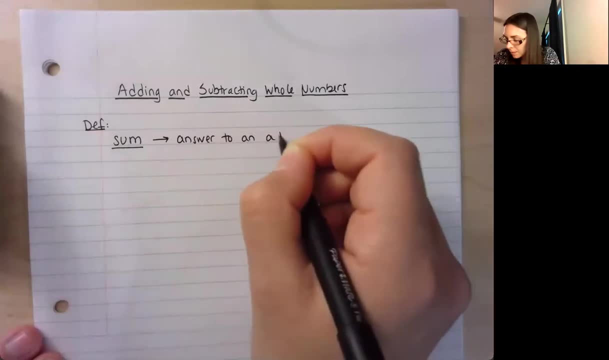 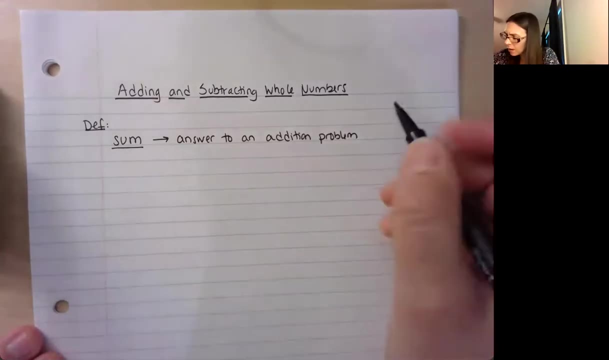 to an addition problem. You can also think of it as well as the total, right? So oftentimes, the sum is also the total if we're talking about an application problem. 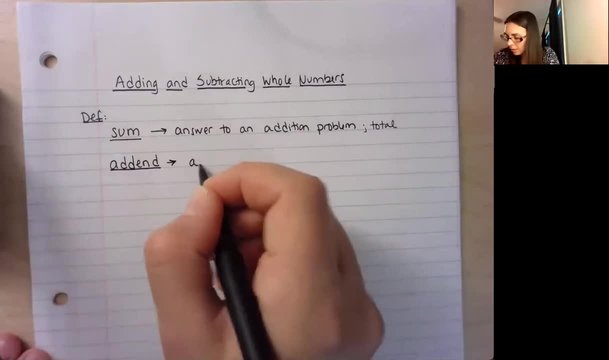 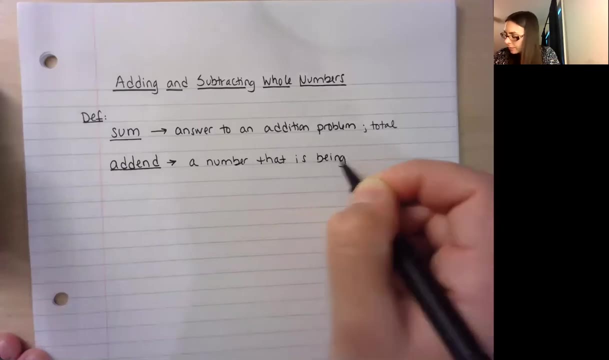 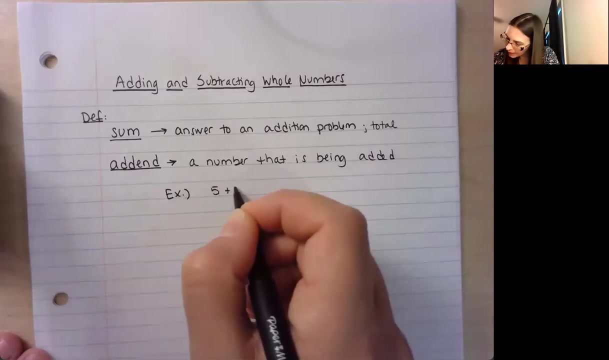 An addend is just a number. So it's just a number that is being added. So as a simple example, let's say you were adding five plus three to get eight. Well, then these here are your addends. This here is your sum. Okay, so it's your answer. 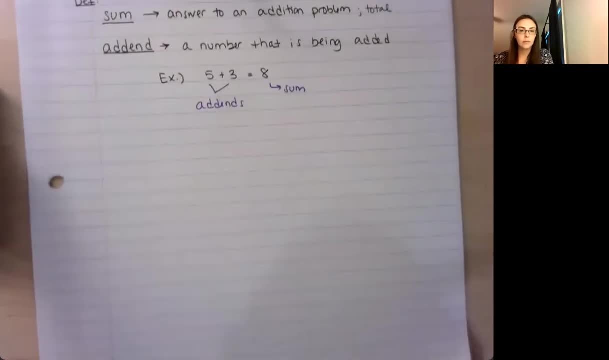 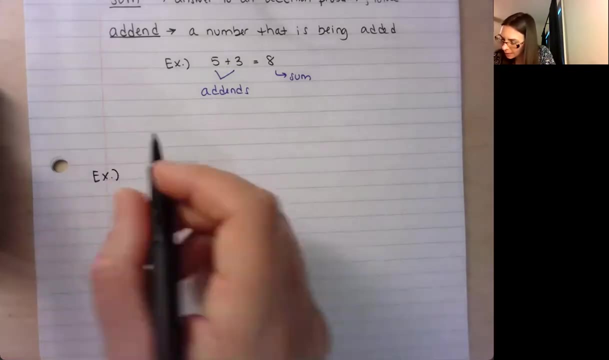 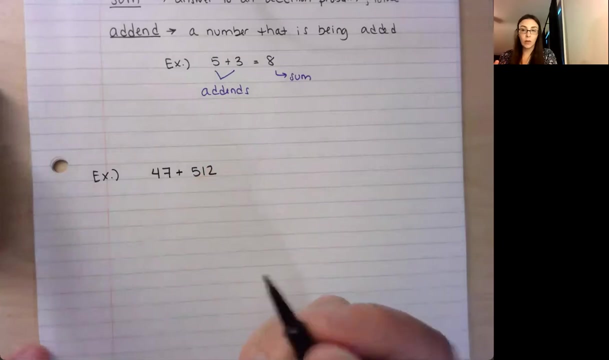 This one says that you've got between 47 and 512. So this is is your answer, and you're going to basically be writing down the sum. You're also going to be adding the rest of the sum to the line. And, you know, once you've added the rest of the sum to the line, you're now automatically writing the rest of the sum to the line. You're going to be adding the remaining sum to the line. So there are a couple of examples. So let's say I want to add the numbers 47 and 512. 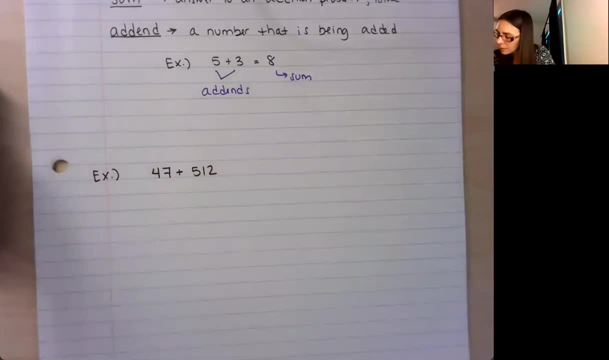 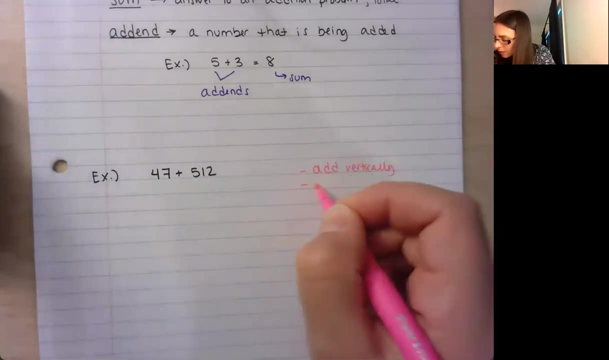 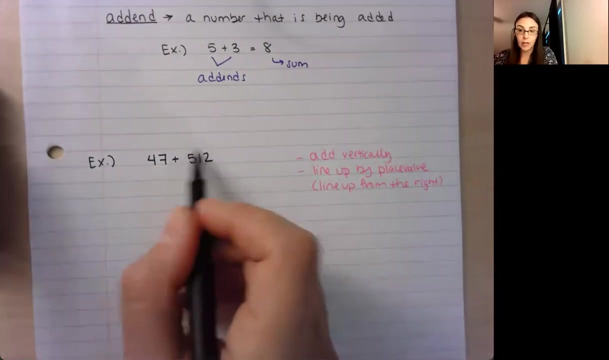 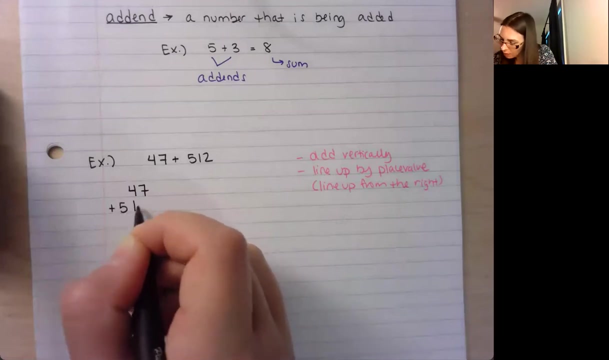 So typically, what we do is we add them vertically. Again, if you're really good at doing arithmetic in your head, then that's fine if you have some different strategies, but I'm going to show you the most common strategies that we're going to use. And for us again, typically, that means we're going to add the last one. we're going to add vertically and you also want to make sure that you line up by place value so you want your place values that are the same place value to line up vertically above each other so think of this as lining up from the right now it really doesn't matter which number you put on the top or the bottom here um a lot of times we like to put the bigger number on top but you're going to get the same answer so you can either write it as 47 plus 512 or if you prefer to write it as 512 plus 47 the nice thing with addition is you get the same answer so whatever works for you and you want to remember that we add same number on top of each other so you can either write it as 47 plus 512 or if you would like to do that you would want to add a column on top of the top which is starting on the right 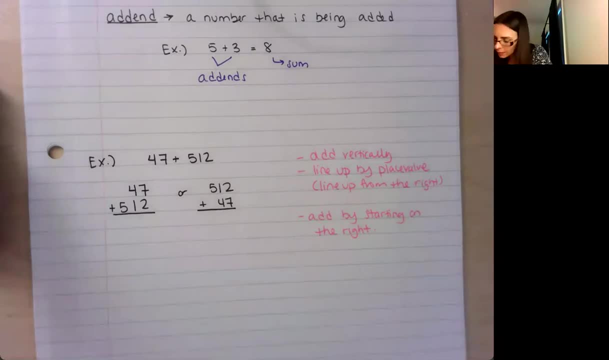 so we're going to add columns here if you find that you make a lot of mistakes what you can always do is use like a light pencil or a different color just kind of those columns nice and organized so i sometimes i find making vertical lines particularly if i have a very long addition problem is helpful just to keep working with it unit conditionally gradient edge area option and all that kind of stuff so thisensitive to end up becoming the bottom drawing.ola to get into the bottom drawinganne to finish this drawing exploring know that starting to set theолот forgess electronic frames and order modules another example you might need to do before you look at our hand out of hand instead of drawing the flip, prof Ges 위해's an old captioner AOT11 card is TACM 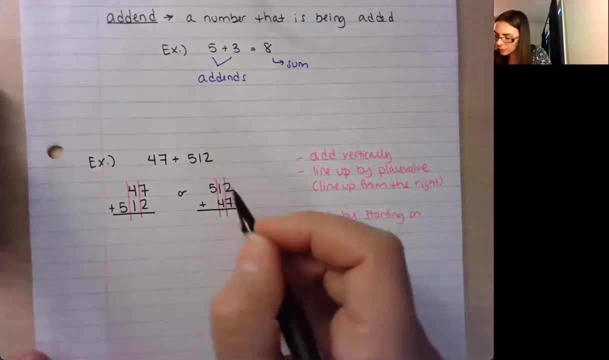 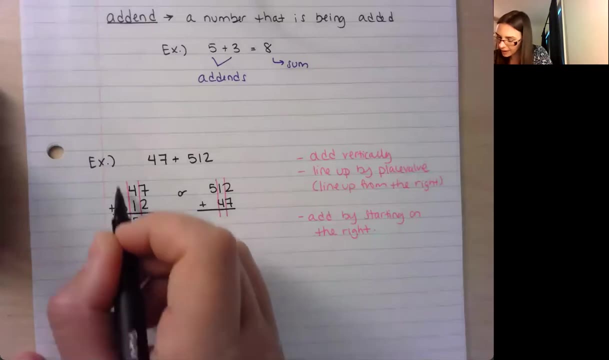 those columns nice and order so here i'll start with this one seven plus two is going to be nine four plus one is going to be five and then if i just have a five i can bring that down on the right you get the same answer two plus seven is also nine one plus four is five 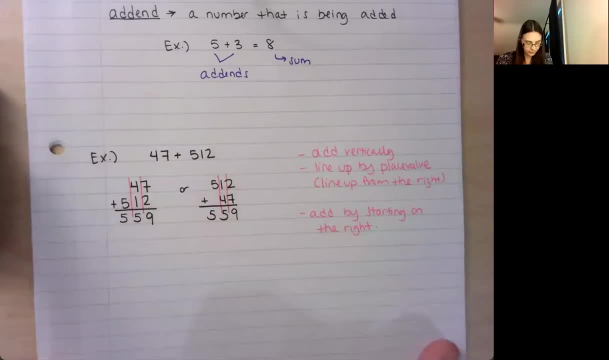 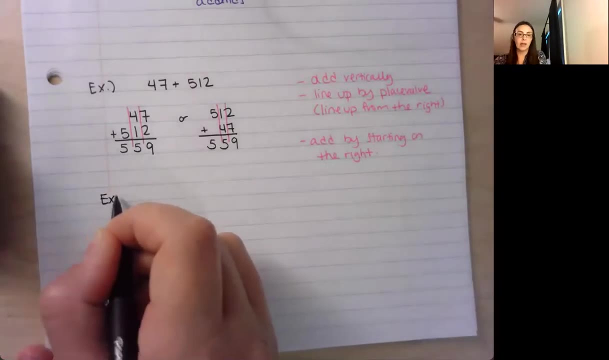 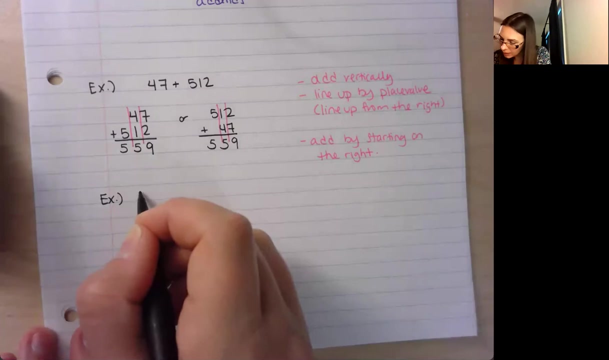 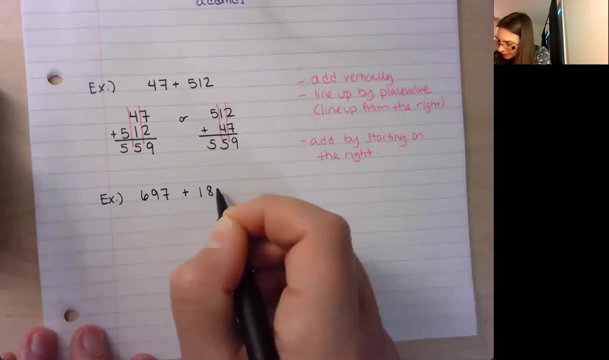 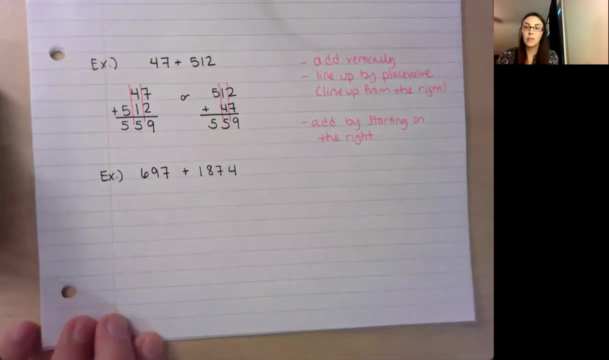 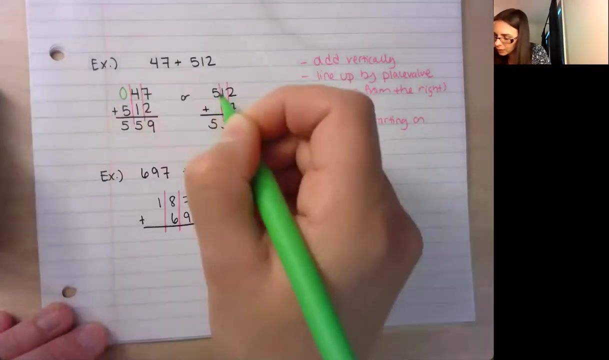 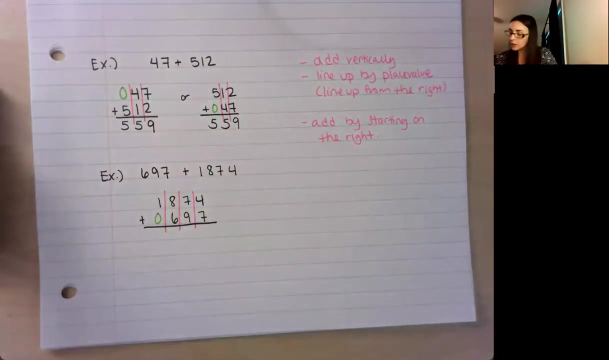 and let's do another example so maybe i want to add let's see how about 697 plus 1874 now again we're going to add vertically i'm going to line up by place value which really means that you're going to line up based on the right so kind of working right to left here same thing when we add doesn't matter what you put first i tend to like my bigger numbers on top so i'm going to do it that way this time i'm just going to make sure i give myself some room here if you find it helpful you can just make some little vertical lines for yourself in between i like to use like a lighter color when i do that just so it doesn't distract me too much this helps me stay organized the other thing you can do although we didn't do the last one is if there's ever a gap you always insert a zero there again if that helps you to stay organized um by attaching a zero it's not going to change the value of our answer so here 7 plus 4 is 11. now this time you're going 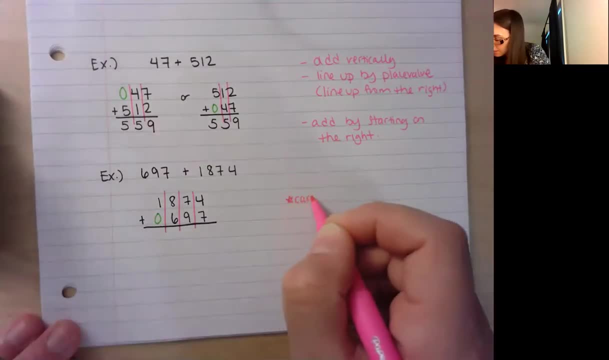 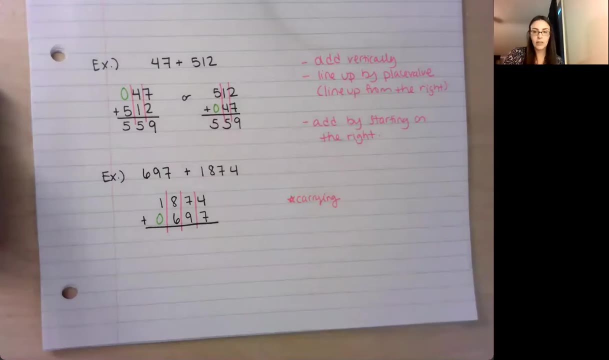 to see something called carrying um which is what happens when you have a value that is more than 10. so again hopefully this is review for you but if not just make sure to follow along carefully 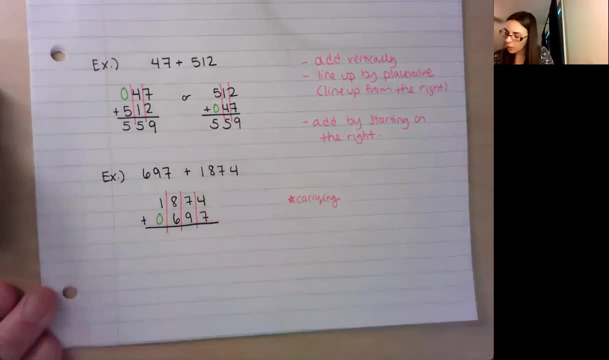 so here 7 plus 4 is 11. so we put the 1 down from 11 in the ones position and we carry the tenth so i carry the 1 from the 10. now i add again so 1 plus 7 is 8 and then 8 plus 9 is going to be 17. so again i put the 7 down in the ones position and i carry the 1 17. so we're carrying the tens position here 1 plus 8 is 9 and then 9 plus 6 is 15. so again i put 5 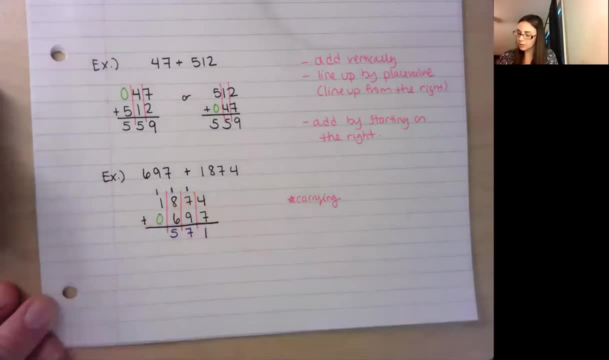 from one's position i carry the tens position 1 plus 1 is 2 plus 0 is still 2. so 2 571 is going to be my final answer 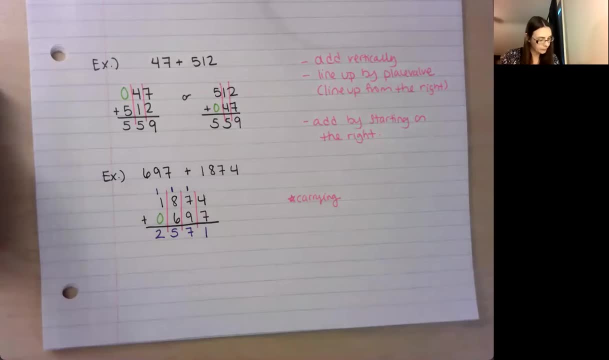 so 2 571 is going to be my final answer all right and let's just do one more example all right why don't we add more than just 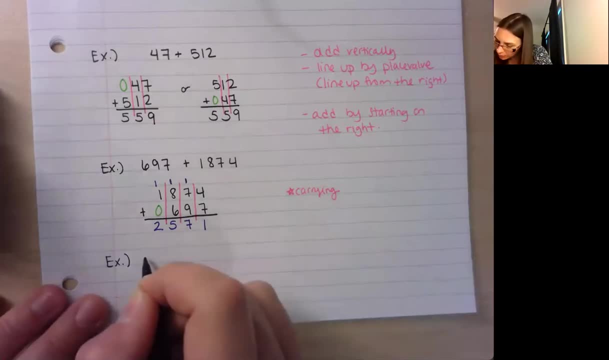 two values this time let's do how about twenty thousand five hundred four plus seventeen thousand nine uh nine plus 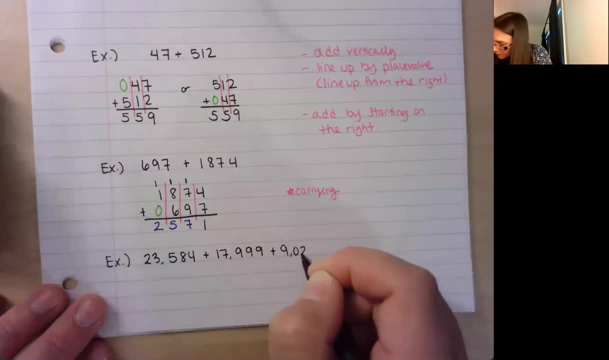 nine thousand and twenty plus how about we do so let's do something a little bit harder 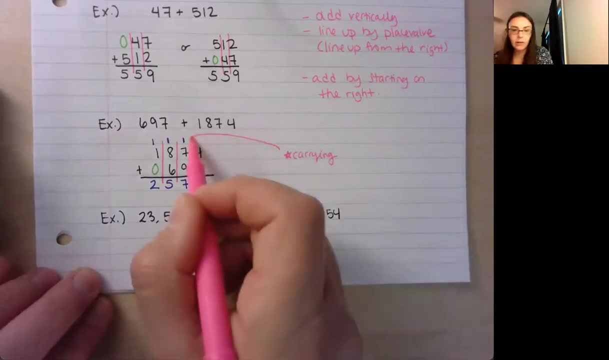 so this is a side note carrying it's this idea right here 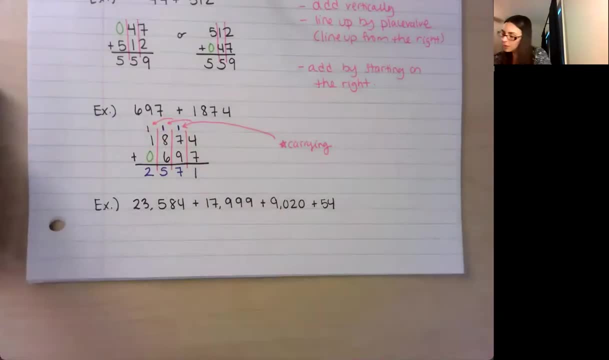 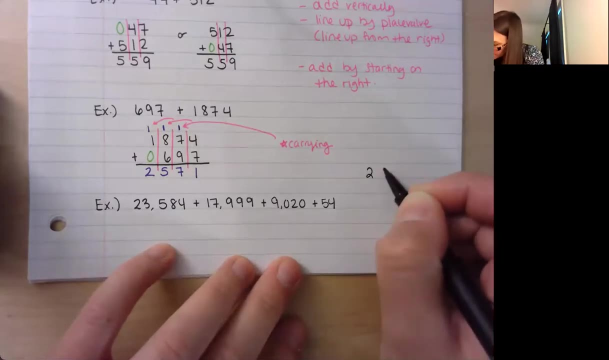 all right so i'm going to make number work over here because it's a much longer number i want to try having enough space so let's see i have two three five eight four and then i have seven three nine nine nine now be careful i'm lining up on the right so nine two oh and then five 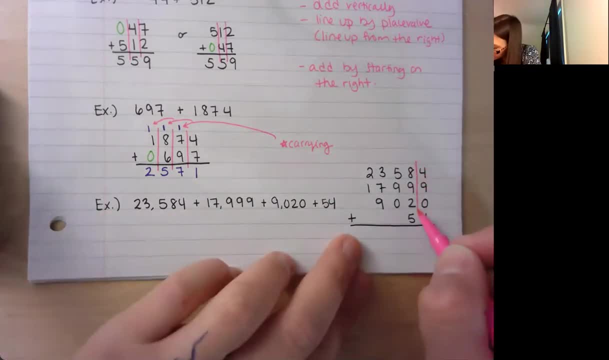 and again if you find it helpful particularly for these harder problems you may just want to draw those vertical lines so you say organize that's all they're for and then i'm going to start on the right working left and then i'm going to start on the right working left 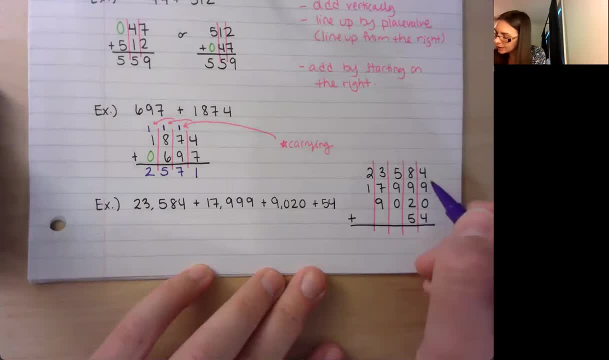 So I have a 4, a 9, a 0, and a 4. 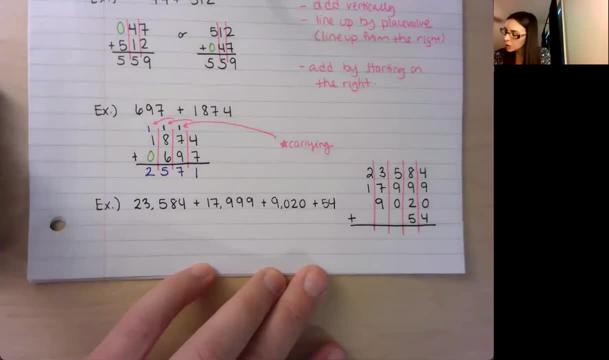 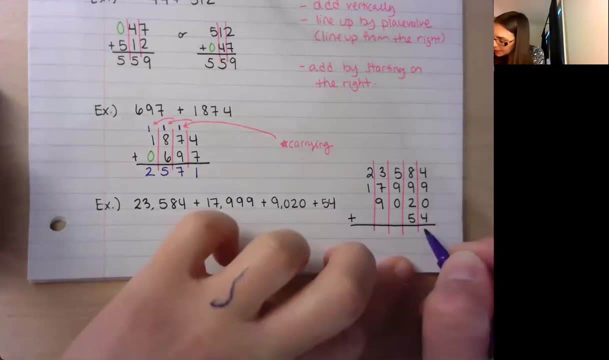 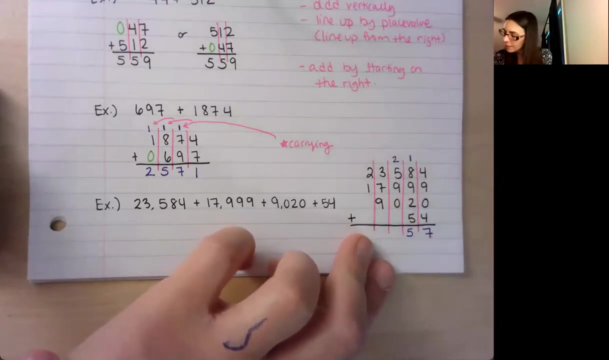 Now when we're adding, we can actually add in any order we want to. So I'm going to do the 4 plus 4 is 8 first, and then plus 9 is going to give me 17. So I put my 7, I'm 1. So again, we always carry the tens position. Here, 1 plus 8 is 9, plus 9 again is a teen, plus 2 is 20, plus 5 is 25. So I put the 5, and I carry the 2 to the tens position. Here, 2 plus 5 is 7, plus 9 is going to be 16. So I put the 6, carry the 1. Here, let's see. 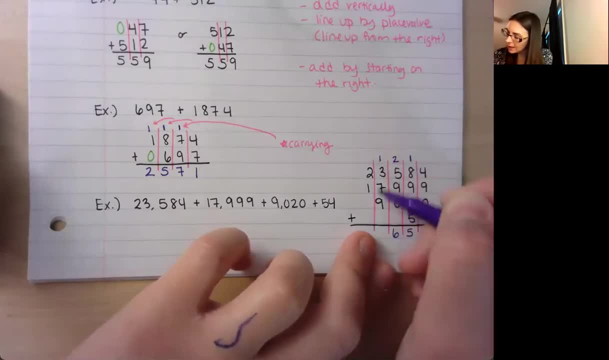 I have a 1, and a 9 is going to give me 10, and then 7 and 3 also give me 10. So I have 20 here. 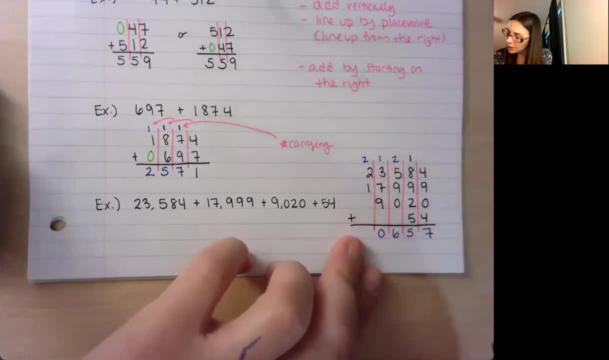 So I put the 0, carry the 2, and then 2 plus 2 plus 1 is 5. 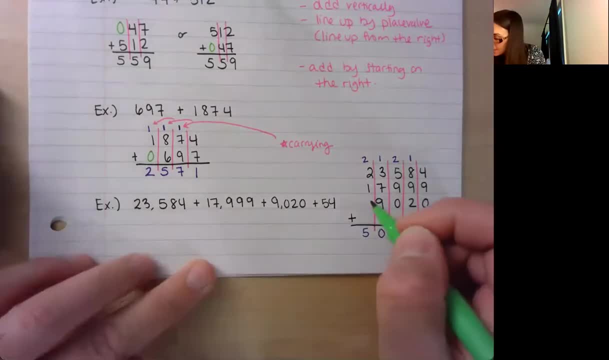 Now again, I didn't do it here because I used my columns to stay organized, but you can always attach or fill in any gaps with zeros if you find that helpful. 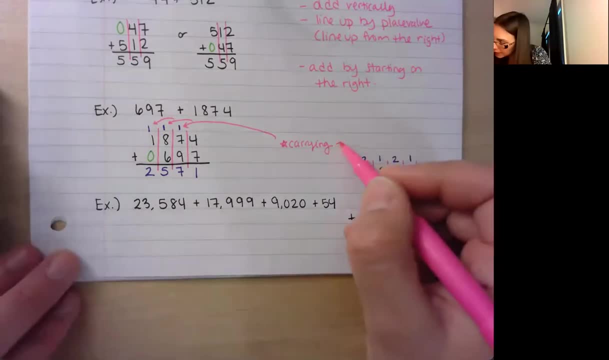 Okay, so again, the idea of carrying when you're just really carrying that position or when we're adding. 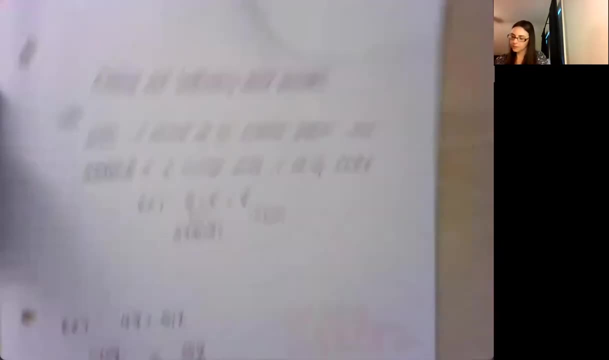 All right, so I have some key properties I do want to talk about for a second. So we're still under the overall heading. So we're still under the overall heading. So we're still under the overall heading. We're still adding and subtracting, but there are some important properties here that we do want to talk about. 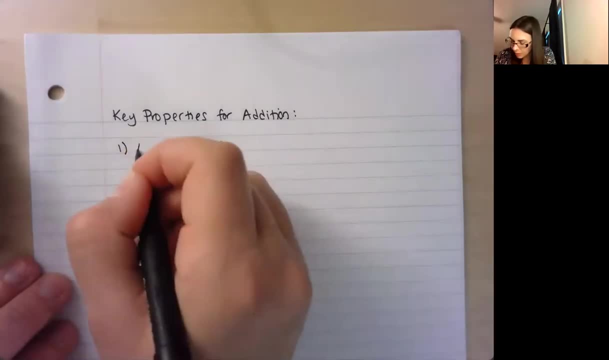 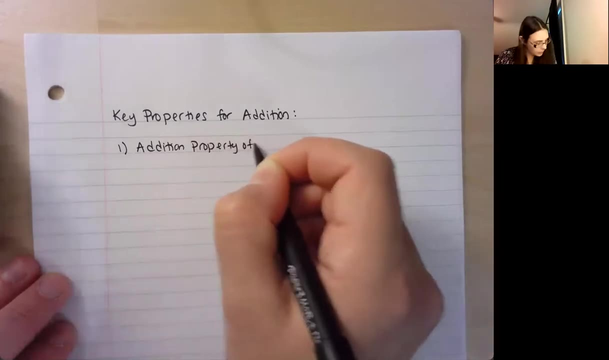 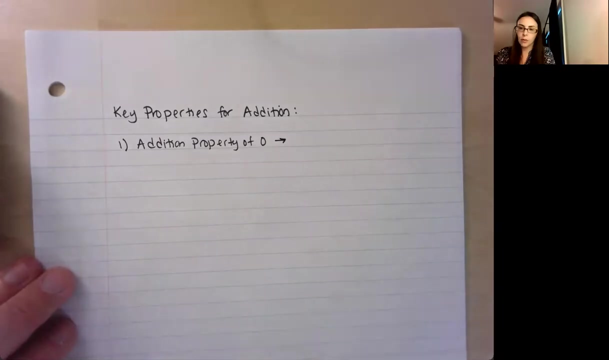 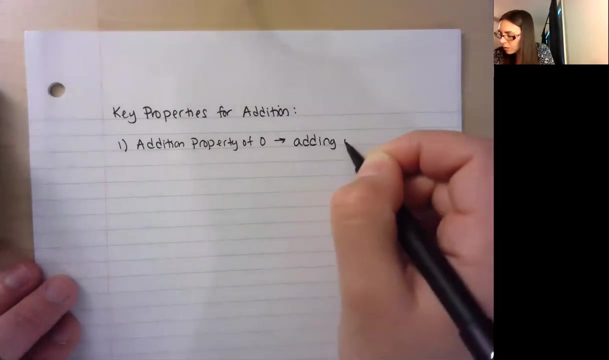 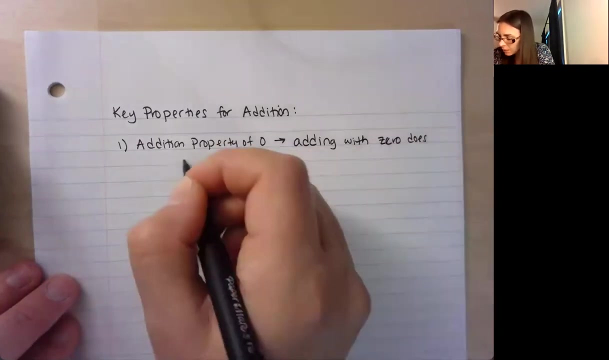 So the first property is the addition property of 0. And basically what it says, and you can kind of read more formally in your text, but what it says is that if we add, so adding with 0, 0 does not change the sum, okay? Which I think everybody knows, right? 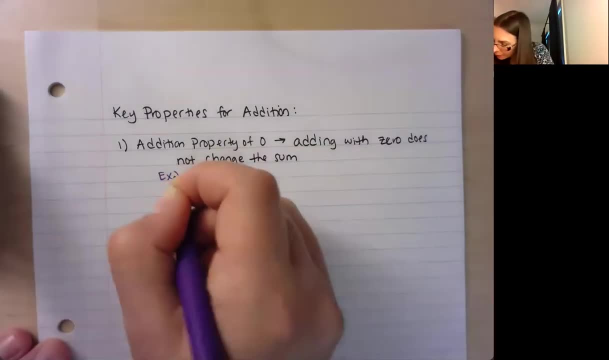 So for instance, 5 plus 0 is still 5. 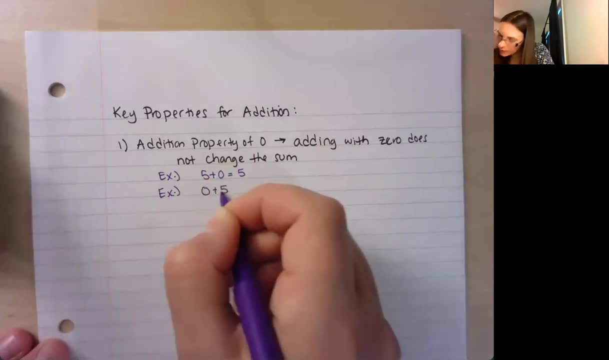 Or if I want to write it the other way, 0 plus 5 is also still 5. So we can add with 0, and it doesn't change anything. 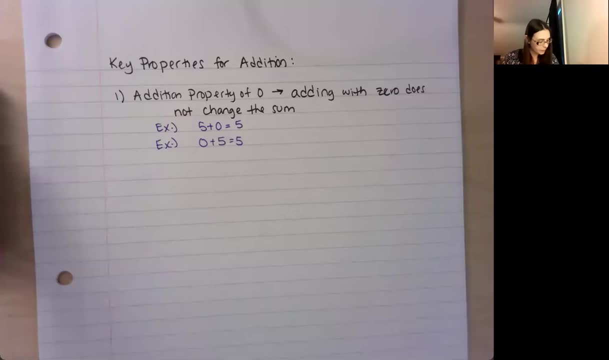 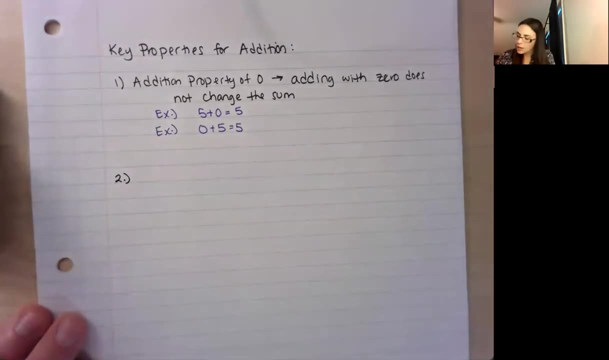 So we're still adding. This is another property that we didn't see nor add before. 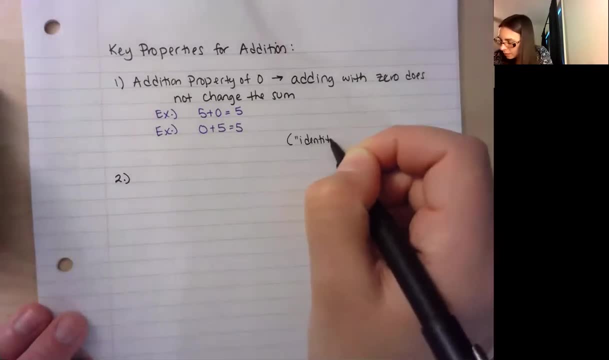 So the number 1 here in our definition of a final group number. If you $1og if you're adding 0. So I'm going to run a daily count feed on this click. This is also a sign that's sometimes called the identity property for addition as well. 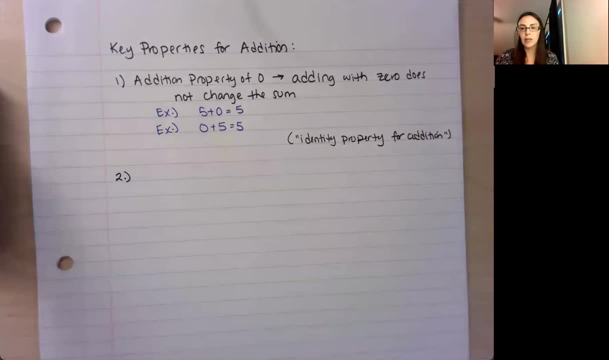 And that's because adding 0 doesn't change the identity of the original number. So that's the salary- 잘�ing account. So you may hear someує This is also a sign that sometimes called the identity property for addition as well. down to 30% is the number. as well. 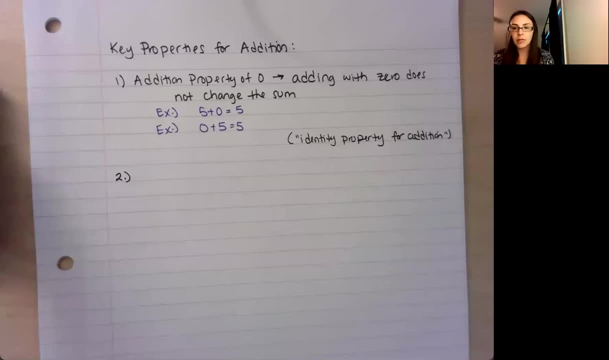 it as the addition property of zero. You may also hear it as the identity property for addition, 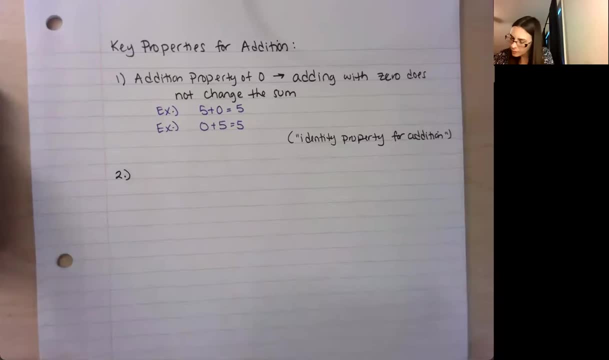 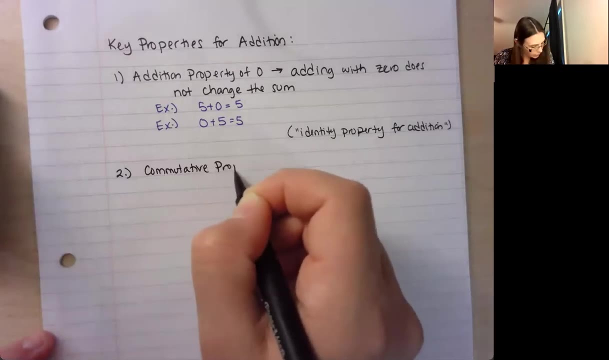 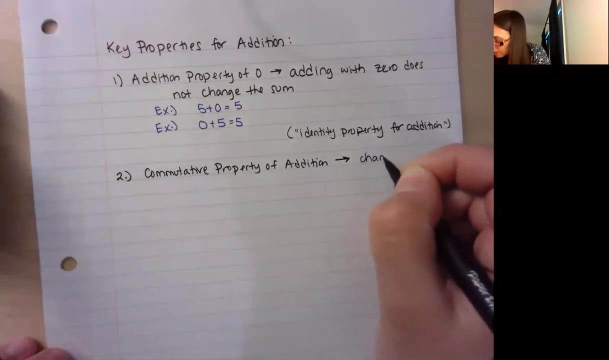 and they both mean the same thing. All right, so the next one is the commutative property of addition, and I've actually been using this already today. And what it says is that it really doesn't matter the order in which you add, you get the same answer. So changing the order of the addition will not 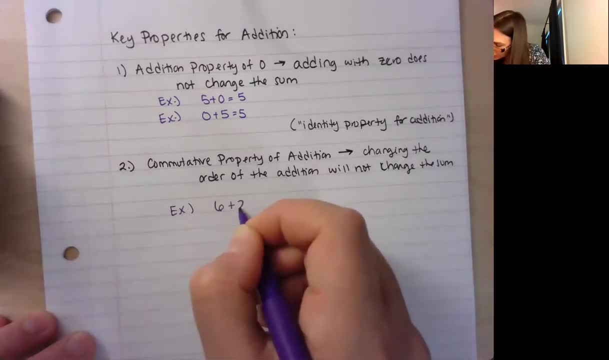 six plus two is equal to eight. 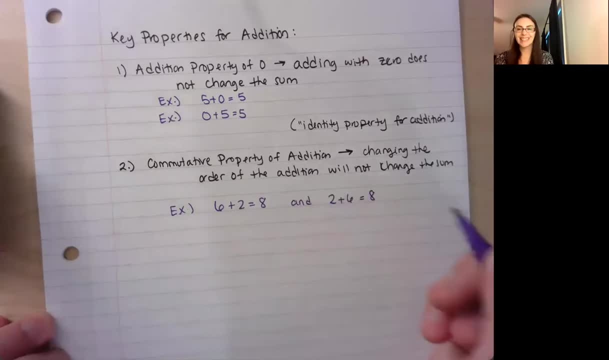 And two plus six is also equal to eight. So we can add in whatever order we want, and the answer is not going to get changed. 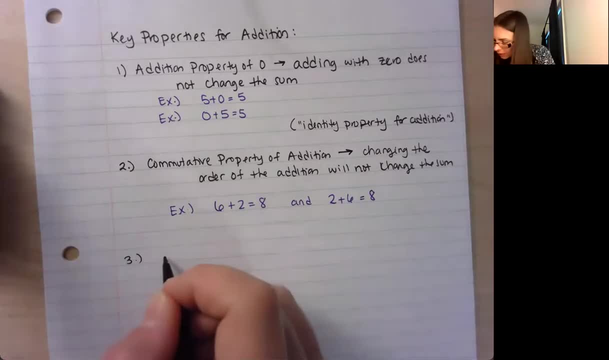 And our third one here is the associative property of addition. 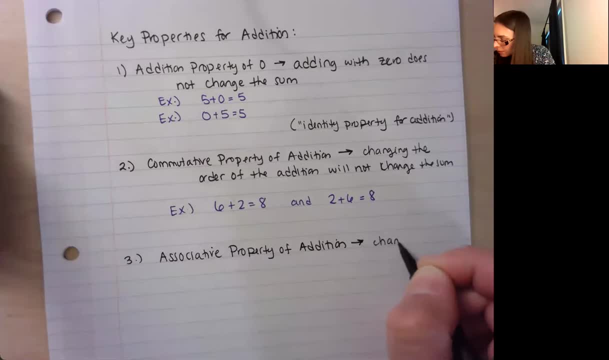 And what this says is that changing the grouping of the add-ins, the numbers being added, and does not change. Again, we sum. So for example, 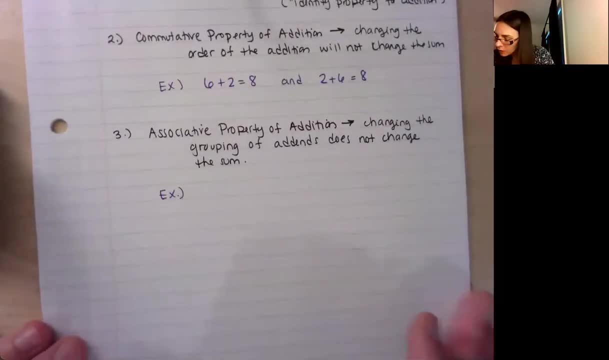 let's say I'm going to bring in parentheses here, so maybe I'm going to add one plus two plus three Well in the first week remember when we have things in parentheses, we have to do that first, so one plus two gets solved first, and that's going to give us three. 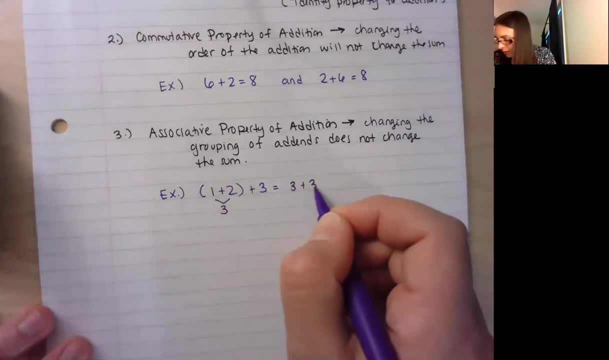 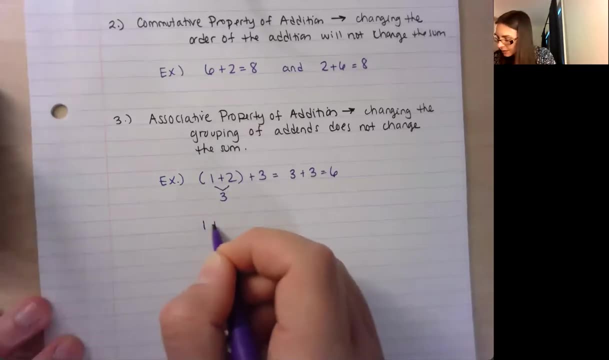 So I end up with three plus three equals two, plus 3, which is 6. Now if I regroup them, maybe I have the parentheses around second two numbers 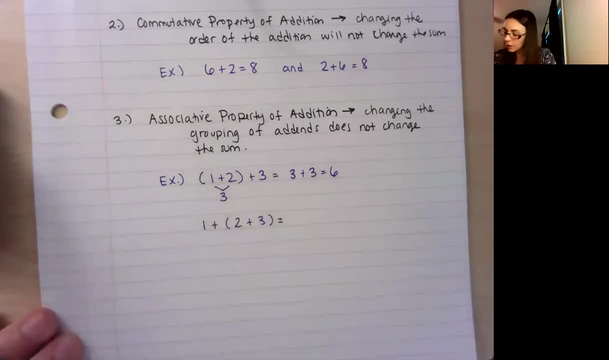 instead. Well, we still would do the parentheses first. 2 plus 3 is 5, but 1 plus 5 is still 6. 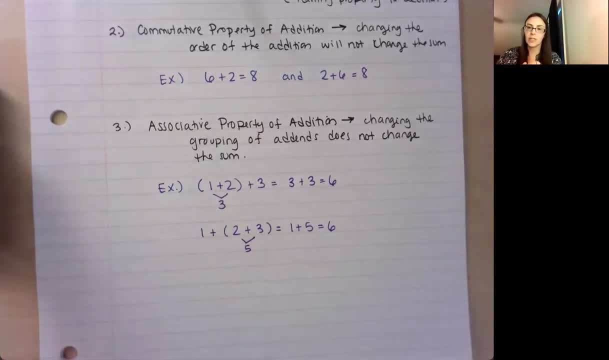 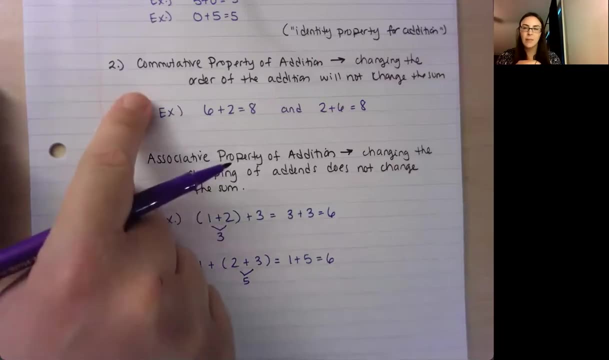 So addition is really, really nice. This doesn't work for everything. So this is actually not going to work for subtraction. But with addition, it's nice because it really doesn't matter the order we add. It doesn't matter how we group things. So you can group things whatever is easiest for you. 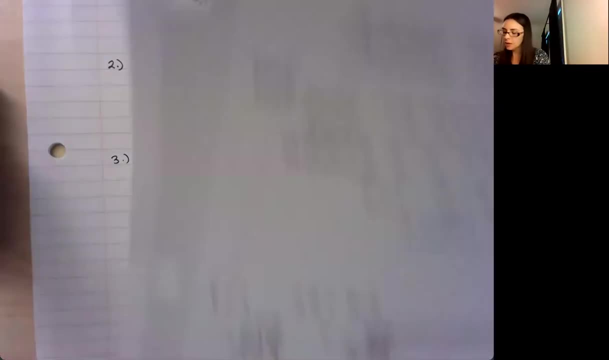 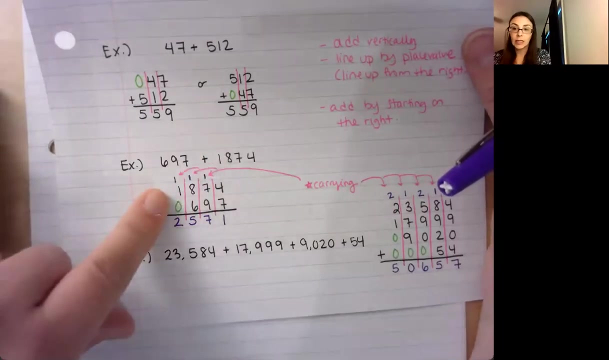 And that's why in the last example, for instance, the last couple of examples, you know, I decided, sorry for this example here, to put the bigger number on top because that was easier for me. And that's totally fine because the commutative property says that I can change the order. 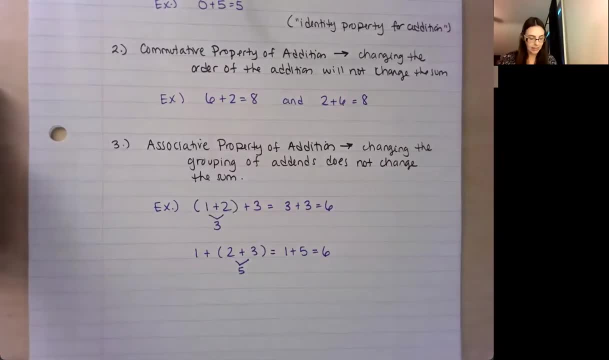 And the associative property says that I can regroup things and do it as whatever's easiest for me. So let's do one more example on this. 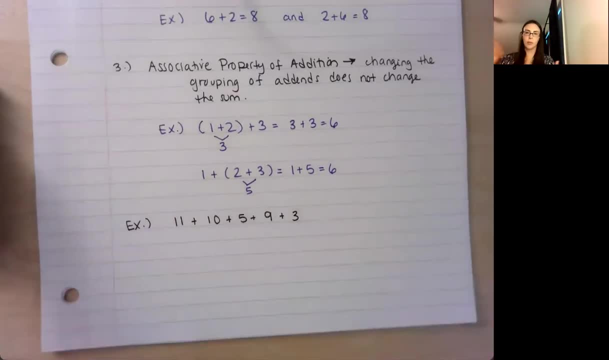 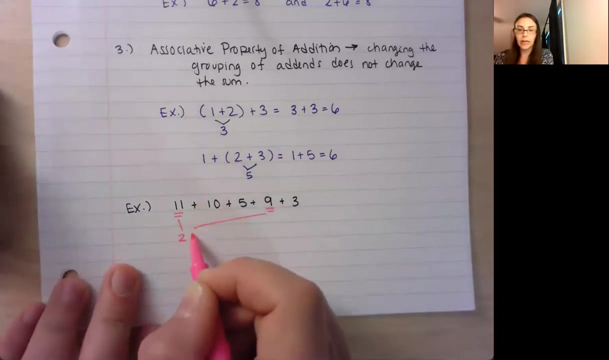 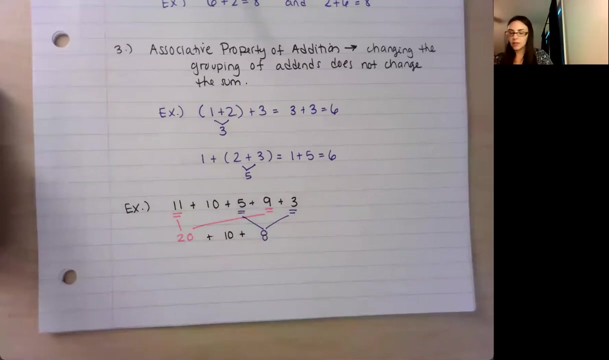 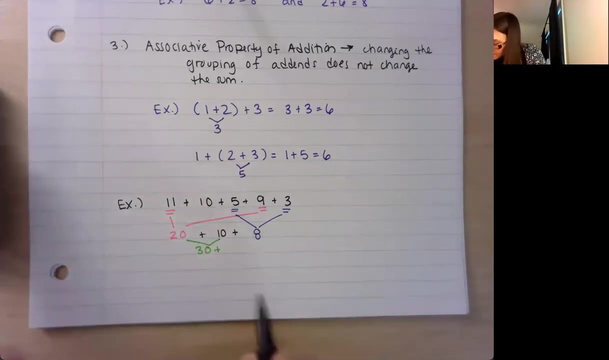 So maybe I have a string of digits that I want to add. And I can add vertically too, but these numbers are pretty small. So you can probably do this mostly mentally in your head. And what we can do is we can just regroup things. So notice, for instance, that I have an 11 and a 9. Now an 11 and a 9 is easy for me to add mentally because 11 plus 9 is 20. So I can just regroup that, kind of rearrange everything using the commutative associative properties and put that together right away. That is 20. Right? And then I can also maybe do, now my brain may work differently than yours. So you may be trying to group these together, my brain is saying, oh, let me group five and the three together because those are both kind of small numbers and that's going to give me eight. And then maybe just mentally, I bring that 10 down for a second. And then for me, the easiest things to do next is to group that 20 and 10 is 30. And then I can quickly do 30 plus eight and get 38. 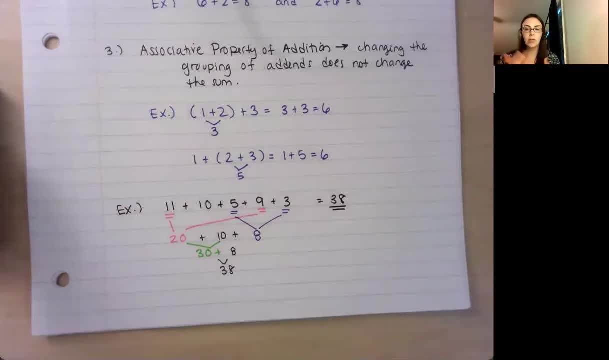 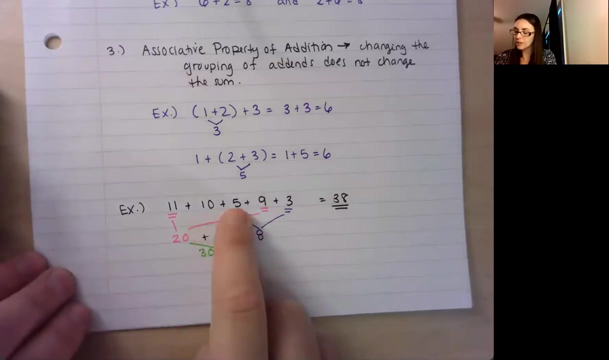 So those two properties really just allow us to regroup. So we can rearrange, to reorganize, regroup, however we want to for addition to make it easiest for us. So you should feel free to do that as well here. And again, you may regroup differently than I did. So you may do like the 10 plus five first and say, well, that's 15 and maybe get 35 plus three instead. So, and that's okay. It's whatever's easiest for you. Okay. So we were talking about how to regroup. 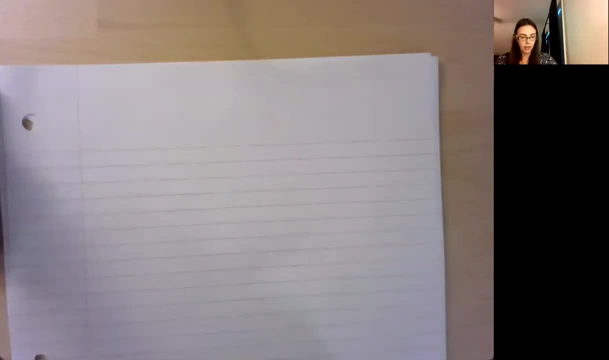 We were talking about addition for a bit, and now we're going to go ahead and move on to subtraction. 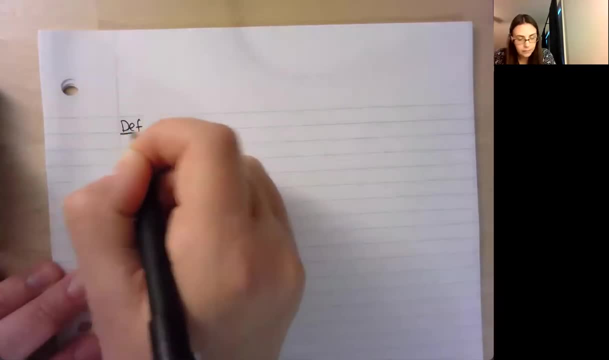 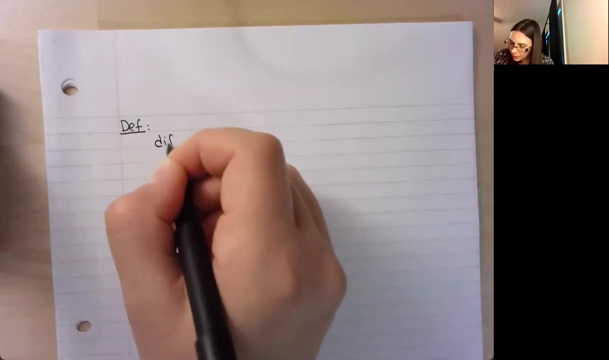 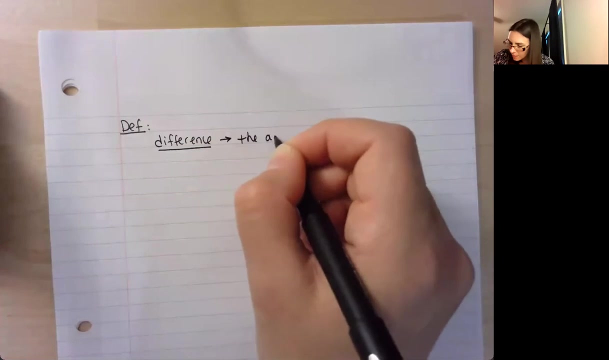 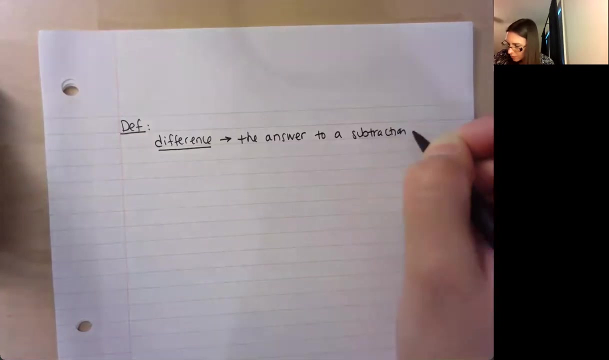 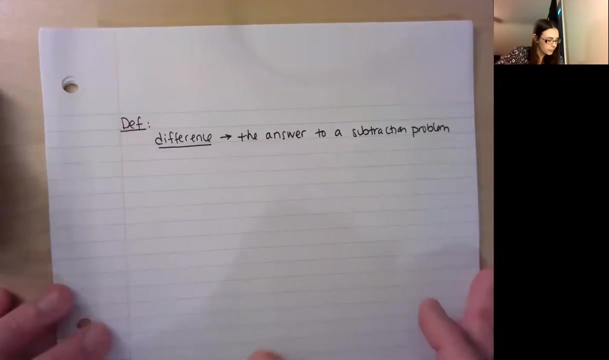 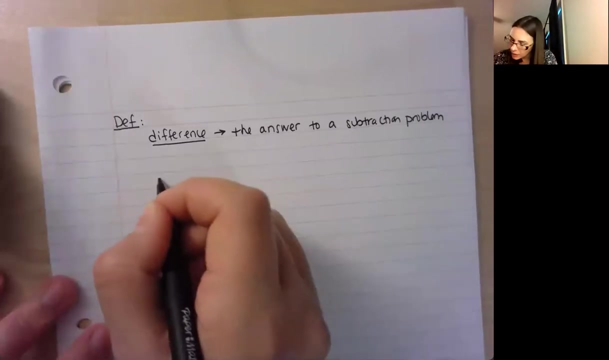 So a couple more keywords here. So we have that word difference. And the difference is the answer to a subtraction problem. So another keyword, just like some differences, a big keyword for subtraction here. All right. I'm going to actually do an example and do a couple more definitions. So let's say we have the example of subtraction. 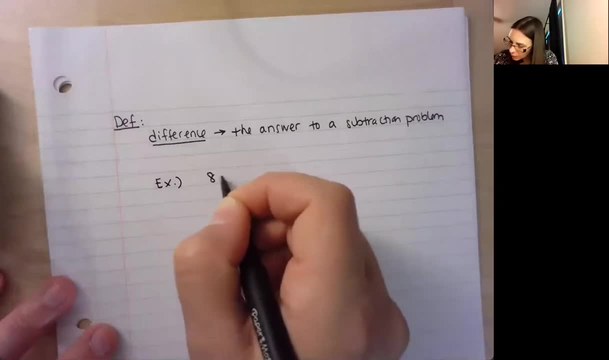 So here is the example. Eight minus three equals five, okay? So five would be the difference here. 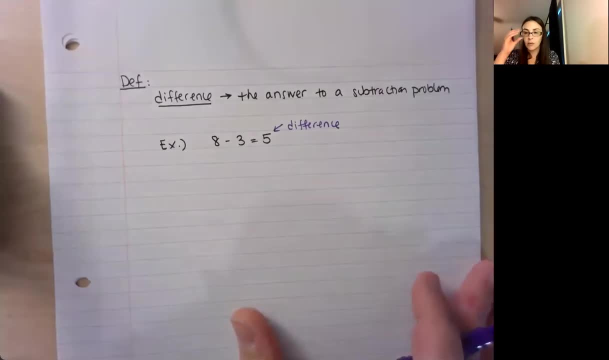 And then we actually have different terms. Instead of using the same term like we did for the addition problems where everything was called an addend, we have different terms for whichever number comes first and whichever number is being subtracted. So the eight here is called the minuend. 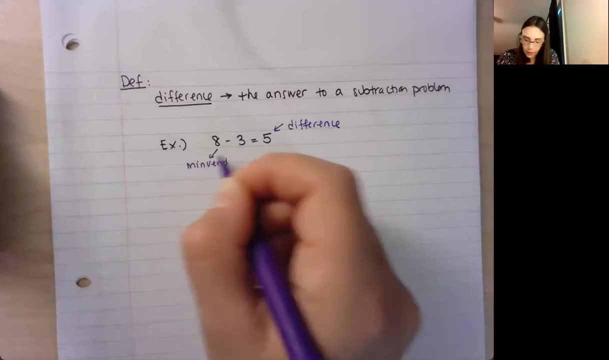 and the three is called a subtrahend. So your minuend is the number that you're starting with, your subtrahend is what you are subtracting, the number being subtracted. 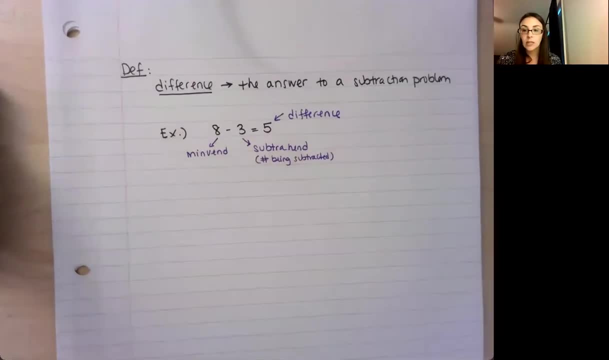 Okay, and again, honestly, I'm not going to use those terms in our lecture. They're really used very, very infrequently, but they are good terms to know just as you're reading through the text or, you know, going through assignments so that you recognize those terms, but realistically, we don't really use them too often. The nice thing is, too, as a little side note here, 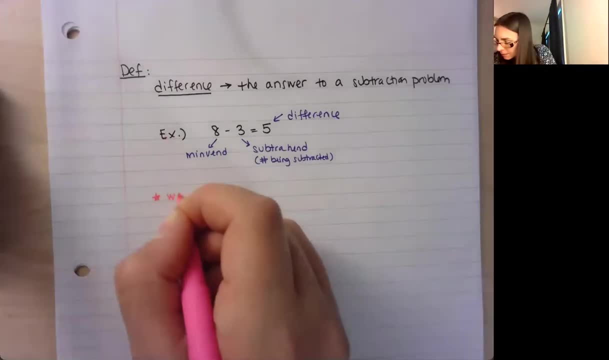 is that we can check subtraction subtraction with addition. 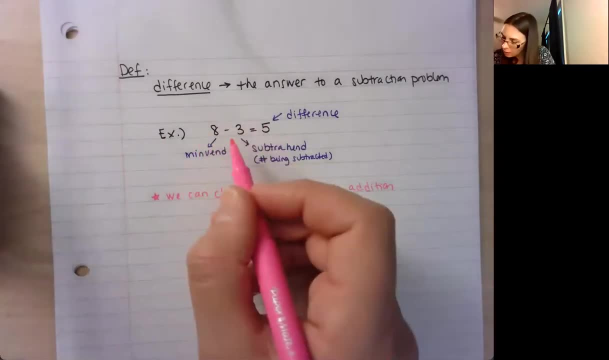 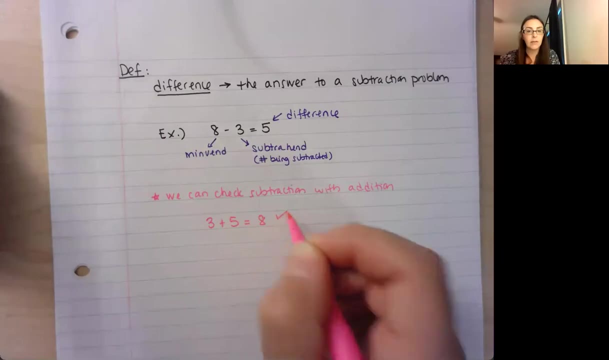 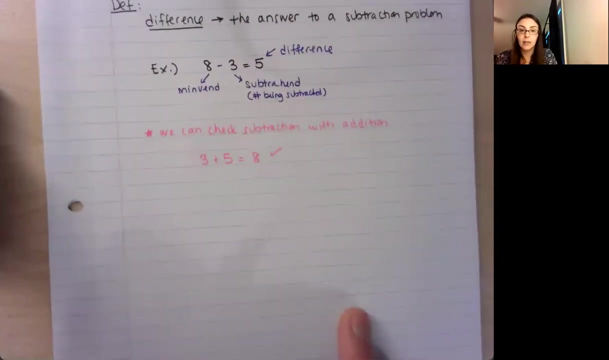 So, for instance, if I'm checking my subtraction here, well, what we could do is I could do three plus five and make sure that it is actually eight, right? So I can check all my answers by using addition as well. So they are directly related to one another. 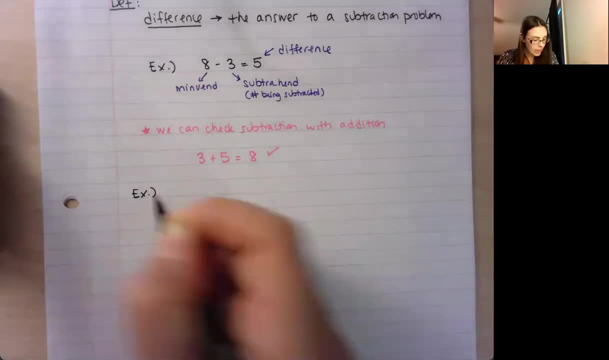 So let's just do one kind of subtraction. Here's an easy example here. So maybe I do something like 20 minus eight. And again, we can do this one mentally. 20 minus eight is going to be 12. 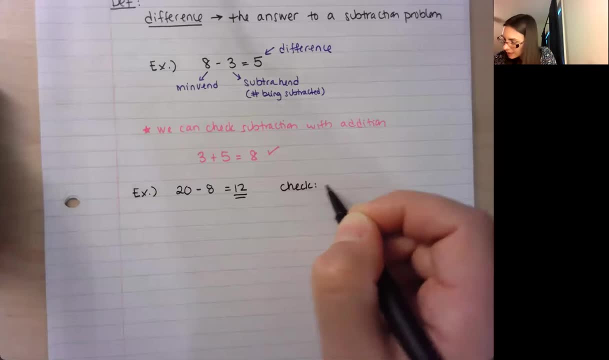 And then to check it, we can check eight plus 12 and make sure it is actually 20. Okay. 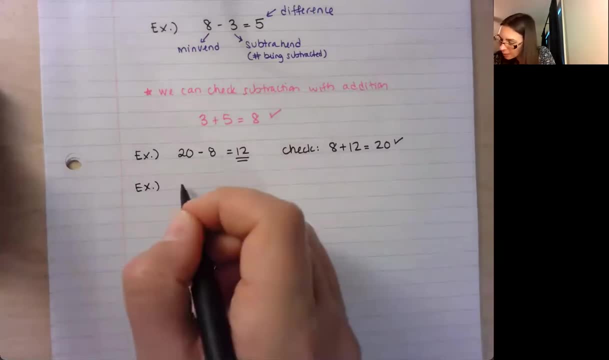 A couple other quick examples. If you subtract the same number with itself, you do, in fact, get zero. 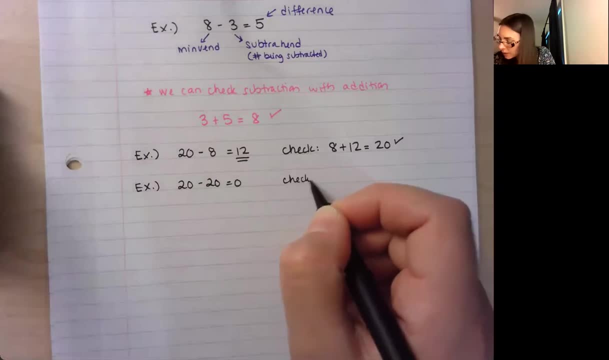 And I suppose you could check this as well, right? If we check this 20 plus zero is still 20. 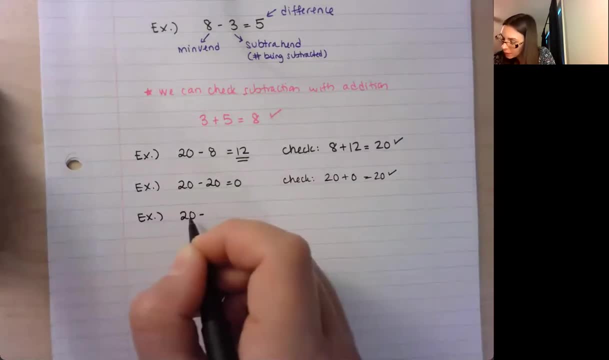 And if you subtract a number with zero, you'll also get that same number. 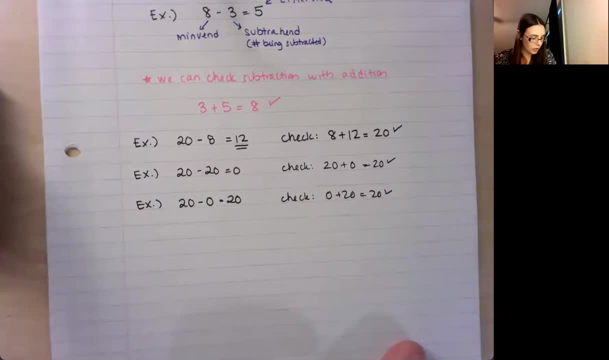 Okay. So just remembering about some zero rules there with subtraction as well. All right. So let's formally define those. 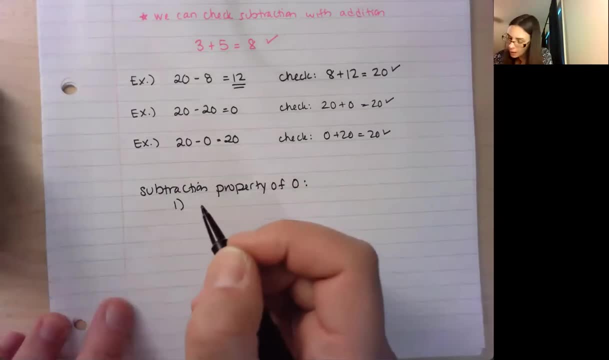 All right. So there's actually two of them that really work together. So the difference of a number and itself is zero. 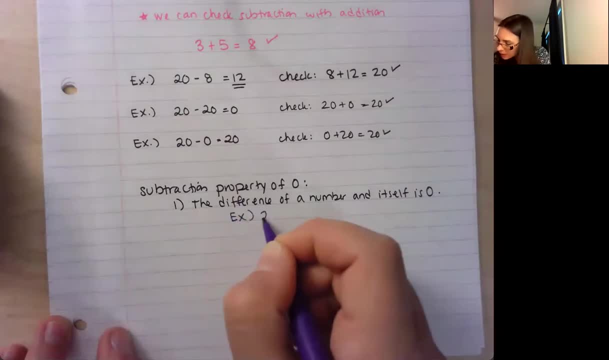 So this is the example we just said about 20 minus 20 would be zero. 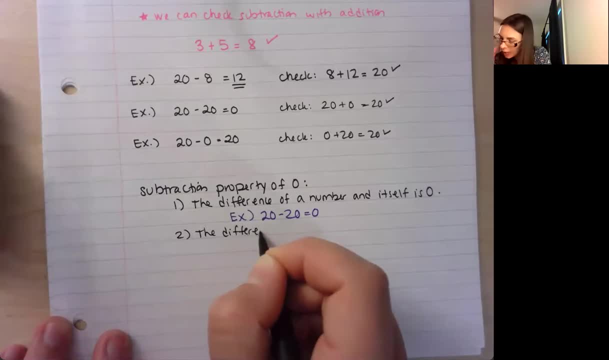 And the difference, remember difference is such a subtraction problem of a number and zero. 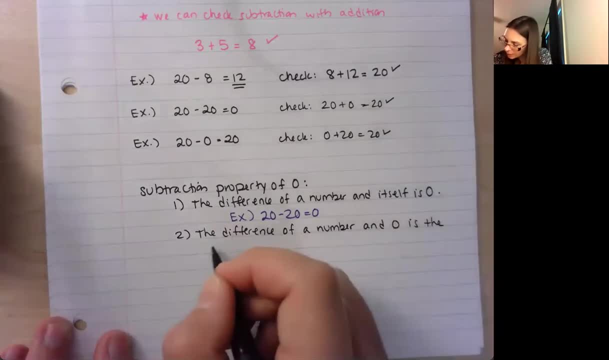 is the same number as the original. 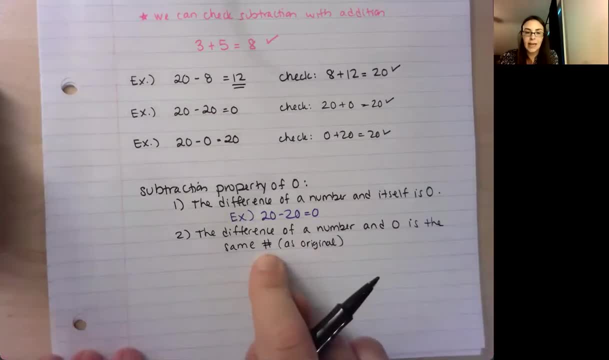 Sorry, this symbol right here also means number, not just hashtag. 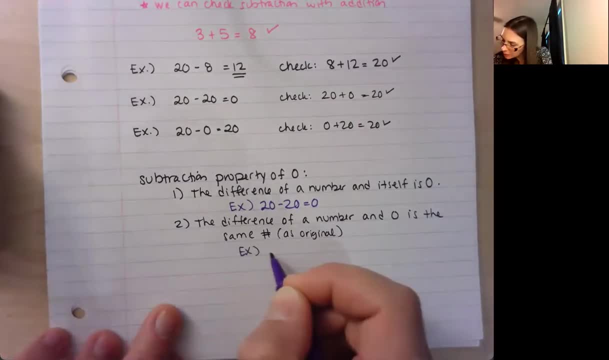 So for example, if I take 20 and subtract zero with it, then my answer is just the original. 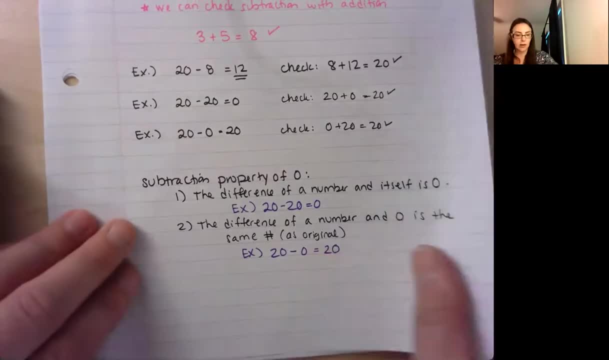 Okay. So let's do a few more examples with subtracting here. All right. 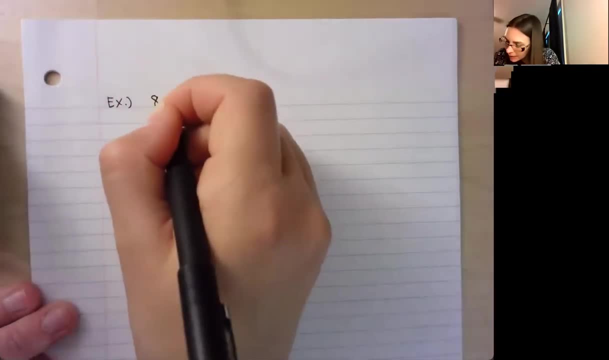 So maybe I have the number 897 minus 542. 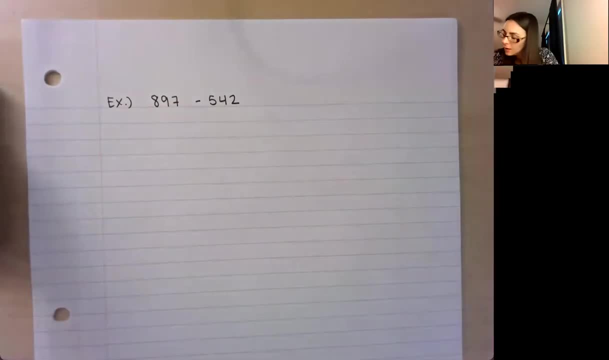 Now, one thing I do want to point out is that subtraction does not have punitive and associative properties. 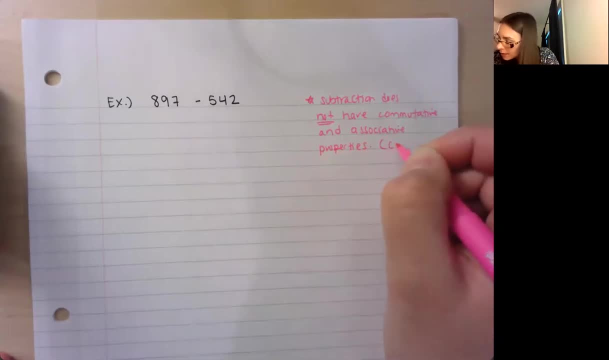 So what this means is that you cannot change the order or read it as you like. 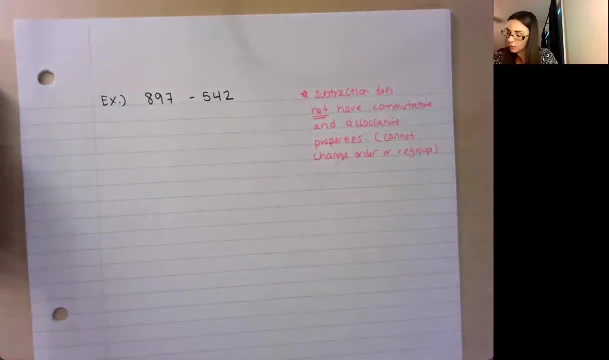 So whatever order your subtraction problem is given in, you have to stay in that order. 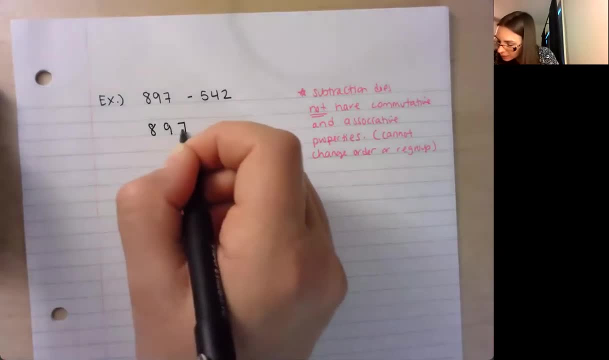 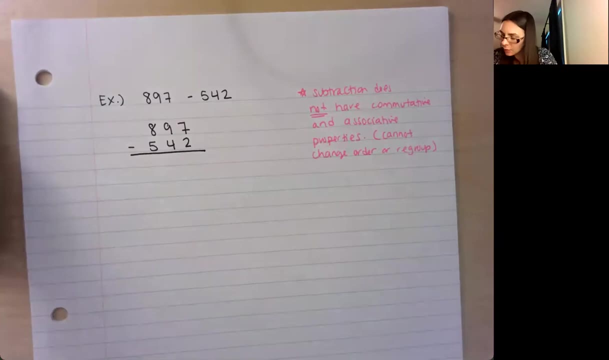 So I have to put the 897 first and subtract it with 502. You're still going to line up the same way. So I'm not going to rewrite those directions, but you're still going to line up just like you would 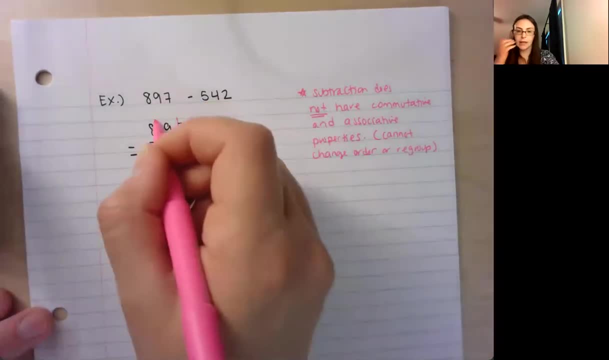 for addition with the same place values. 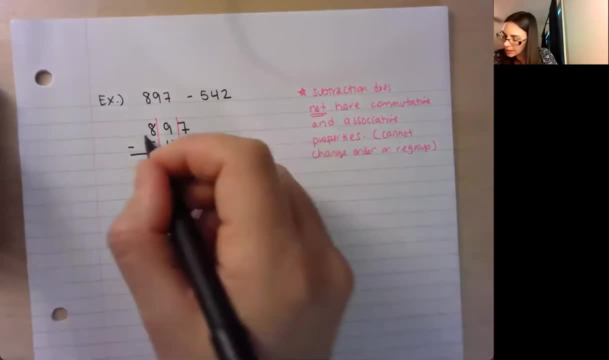 And then we're going to go ahead and subtract. From the right to left. So 7 minus 2 is 5. 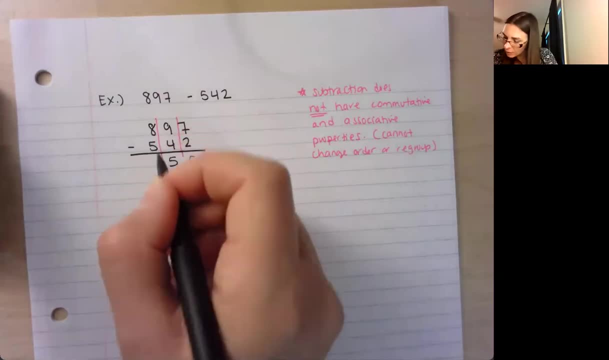 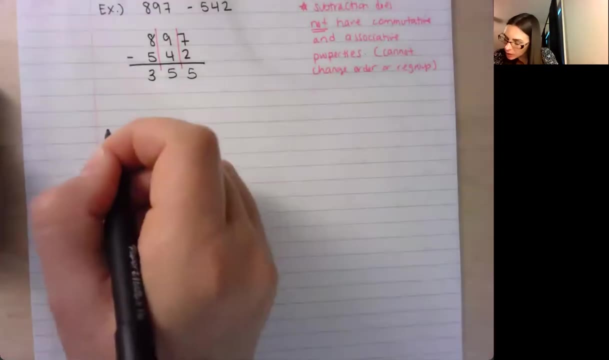 9 minus 4 is also 5. 8 minus 5 is 3. Sometimes with subtraction, you may have to also borrow, just like we kind of had that carrying idea. So let's try another example. 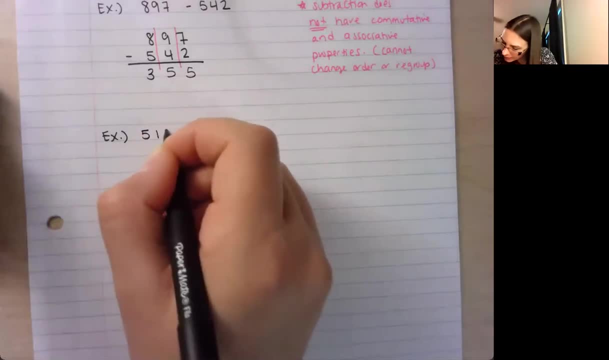 Maybe I have 518 minus 489. Okay. 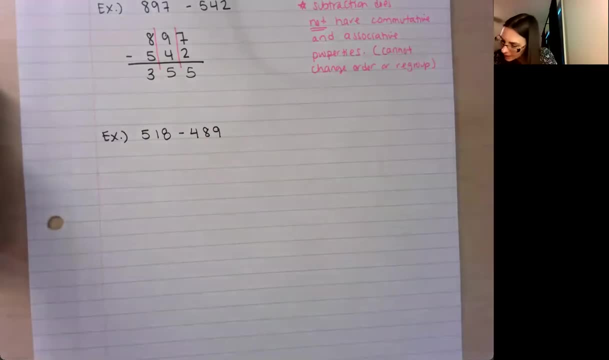 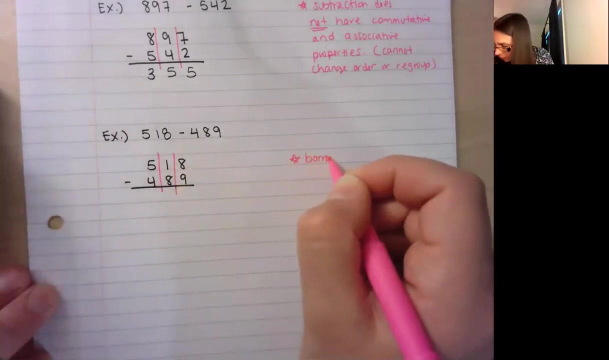 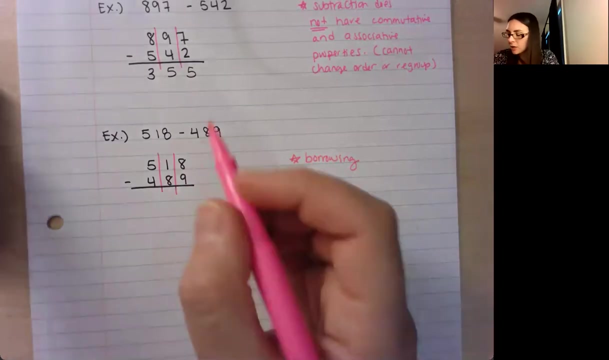 So I'm going to stay in order. And just line everything up like I did with addition. And just don't forget, sometimes we have to borrow. So we have to borrow. Again, we're using tens here. So I try to do 8 minus 9 and I can't do it. 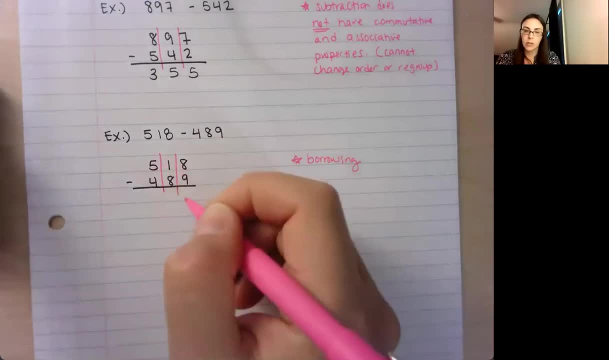 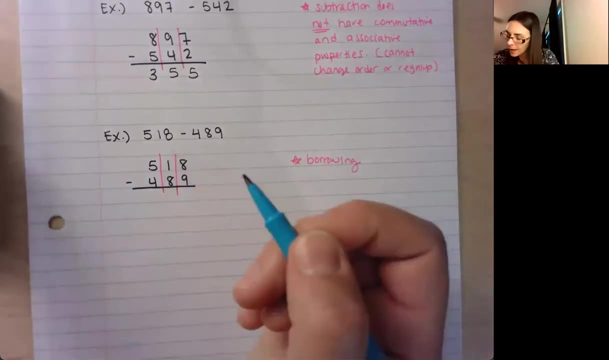 8 is not big enough, right? It's not going to be 1. You can't subtract backwards. So 8 minus 9 is not big enough. So what I need to do is I need to borrow. So I go over only one space at a time. And I take 1. So I'm going to take 1 from here. So that 1 becomes a 0. 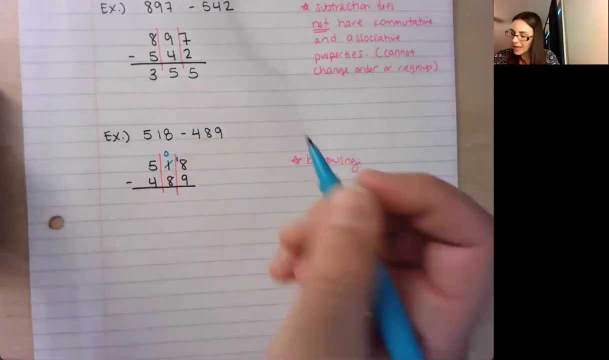 And then I bring that 1 back over. So this 8 actually becomes an 18. 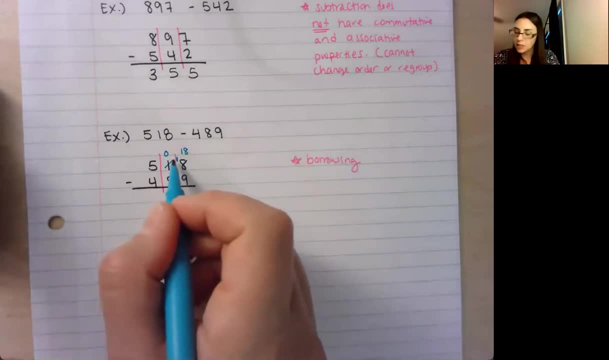 Now you can either write it like this if you're good at doing subtraction. Or if that's too tricky, then just cross it out and rewrite it as 18. Whatever is easier for you. 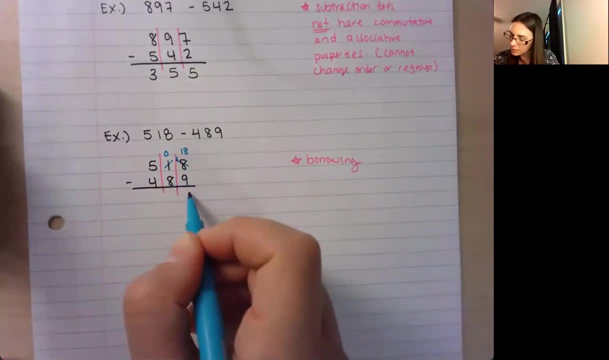 So now I can do 18 minus 4. I can do 8 minus 9, which is 9. I cannot do 0 minus 8. 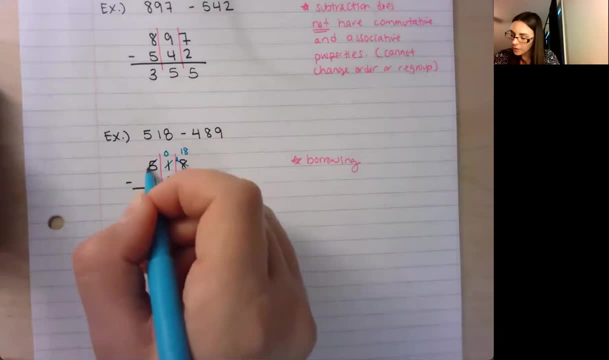 0 is too small. So I go over one spot. I borrow one unit from the 5. Make it a 4. And then that 0 is going to get a little 1 added on front. So 0 becomes a 10 here. 10 minus 8 is 2. 4 minus 4 is 0. So if you want to put that down initially, you can. 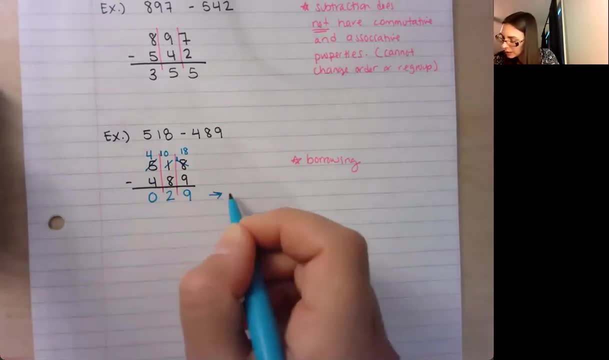 But we don't need leading 0s. So our answer here is just 29. Okay. 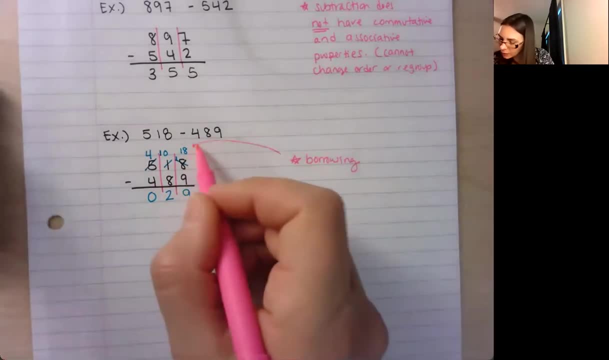 So borrowing is this idea right here, where we're taking from the next digit over. 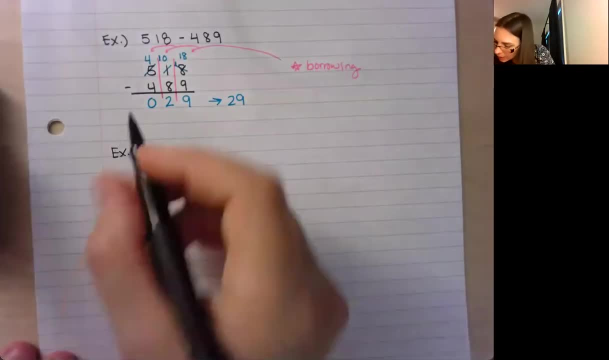 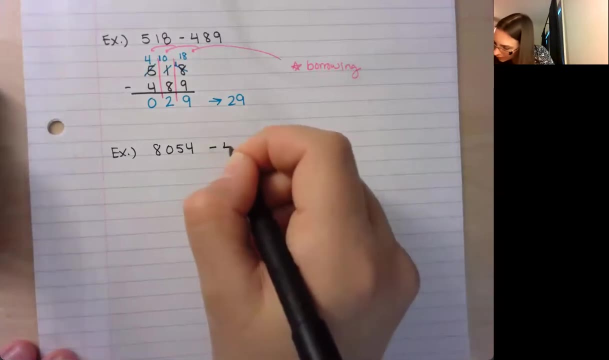 Let's do another example. I'm going to do 8,054 minus 4,902. 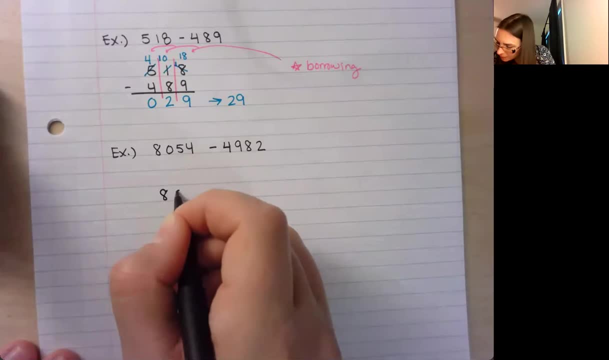 So I'm going to line everything up first. Just staying organized and giving yourself enough space is actually probably one of the most important things. 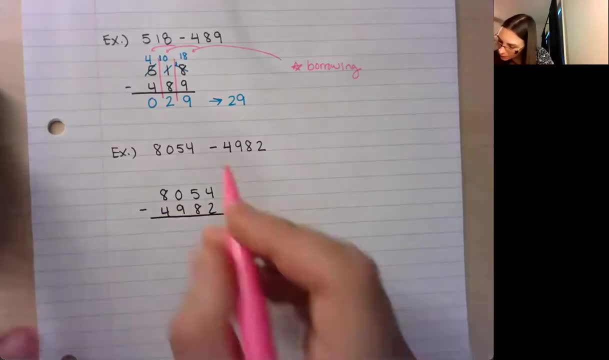 A lot of students make mistakes just because they're being messy. Or they're trying to write their answer on a tiny scrap of paper or something like that. 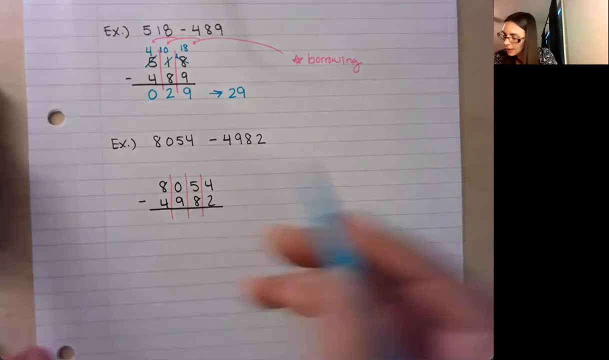 So stay nice and organized here. Now I start right to left. So I do 4 minus 2, which is just 2. So if you can subtract, you just subtract. You don't always have to borrow. Here, 5 minus 8 is 2. 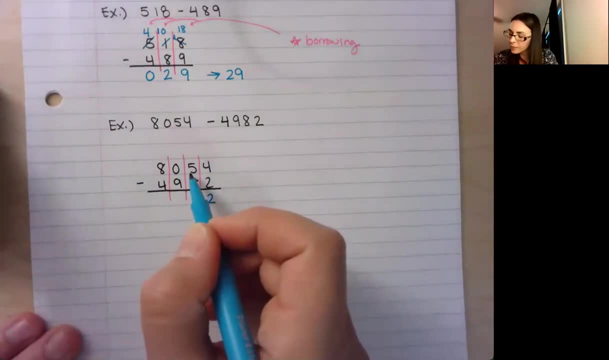 Here, 5 minus 8, I cannot do. 5 is too small. Now I go to borrow the next spot over, but I don't have anything there. 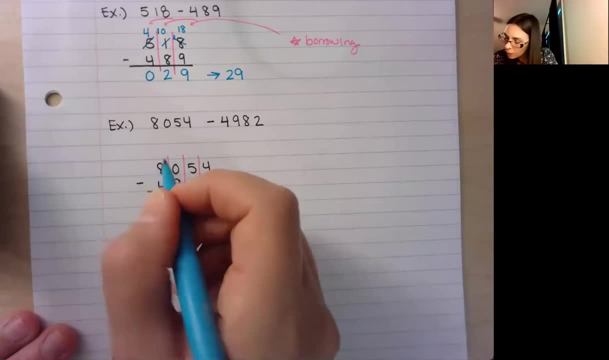 I have a 0. So I have to go one more spot over. Now whenever you're borrowing, you work backwards one little place at a time. So the 8 becomes a 7. 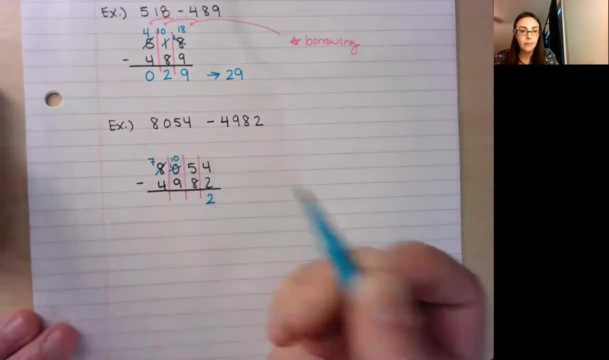 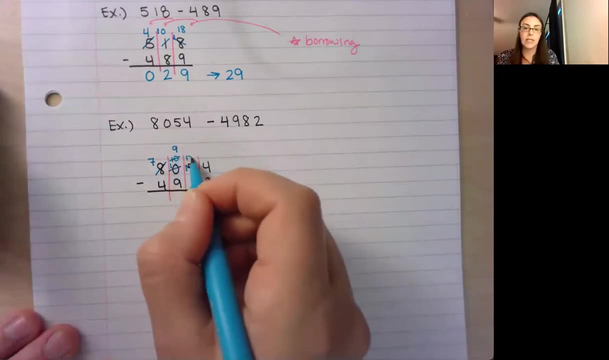 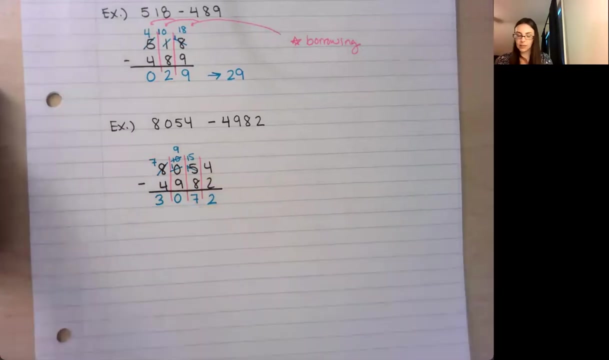 And then this first 0 becomes the 10. Now I can take from the 10, make it a 9. And my 5 here becomes the 15 I need. So when we borrow, you can't jump. You have to go one spot at a time. 15 minus 8 is going to be 7. 9 minus 9 is 0. And 7 minus 4 is 3. So I have 3,072. 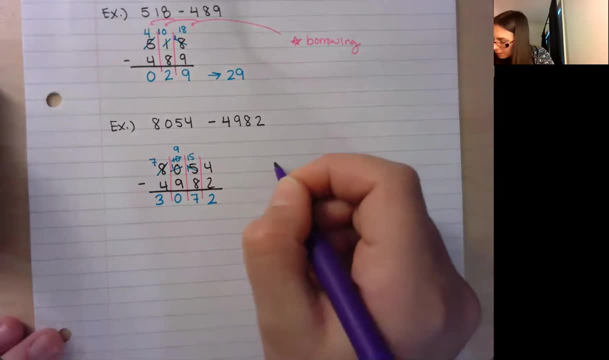 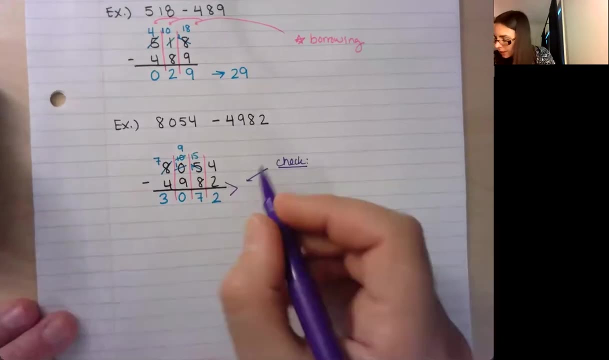 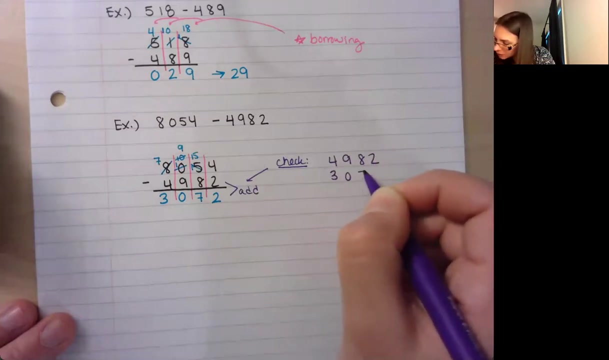 Now let's actually do a quick check here as well. So when I check, I'm just going to go ahead and add these last two values to make sure that it works. So I would take that 4,902. Add it with the 3,072. I get 4, 15 times 1, 10 times 1, 8. And I can see that it does actually match my original value. So it does check out. And you can check any of your subtraction problems. 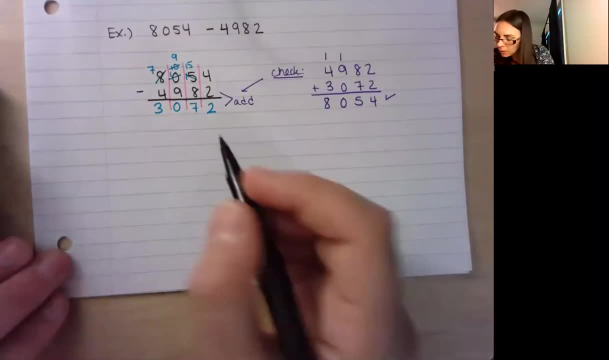 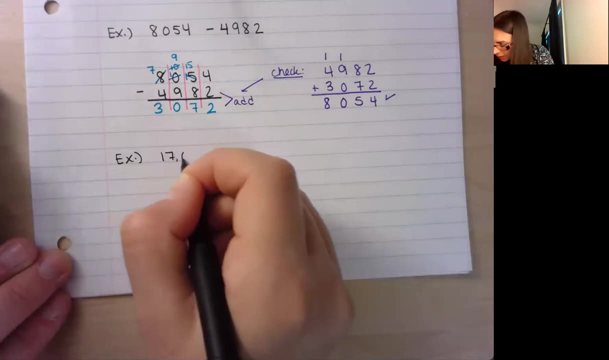 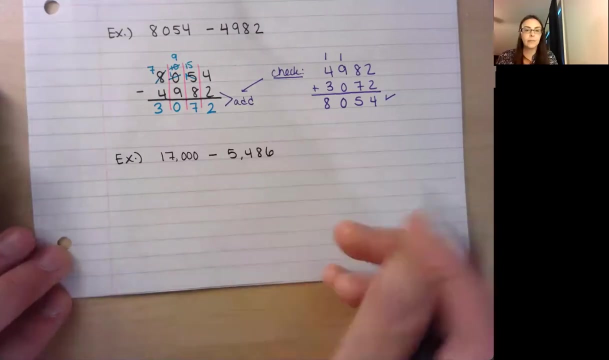 So I'm not going to check any more of them. I'll just check that one to show you. And I'm going to do one more example here. So let's do 17,000 minus 5,406. All right. So first thing is to line everything up. 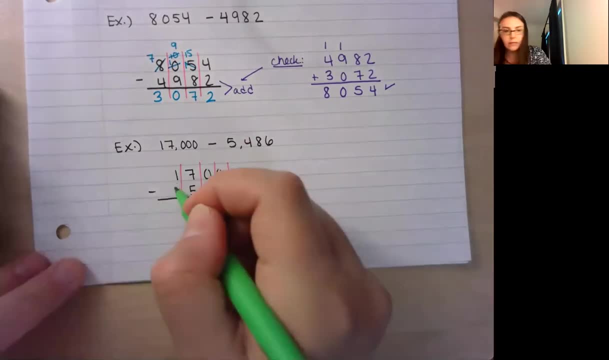 Now, again, if you want to, you can always insert any zeros. If you have missing values, that may be helpful for you. When you're subtracting, though, with whole numbers, your bigger number does need to be on top. 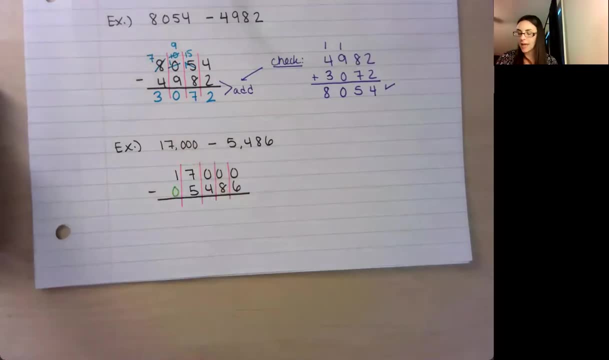 So it should be given to you in the correct order so that you can line everything up like this. All right. 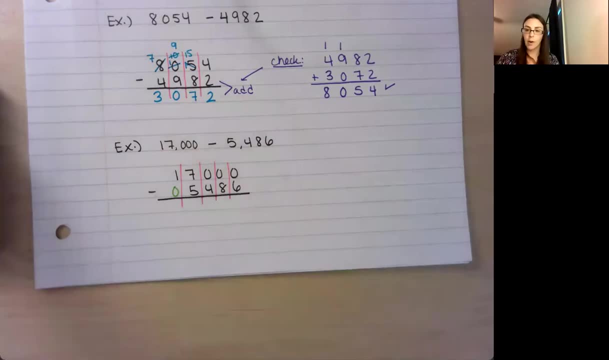 Now, in this case, I'm going to try to subtract, and I have to do a lot of borrowing. So I try to do 0 minus 6, and I can't do that. I need to borrow. I go to the next digit, and it's still 0. Next digit is still 0.